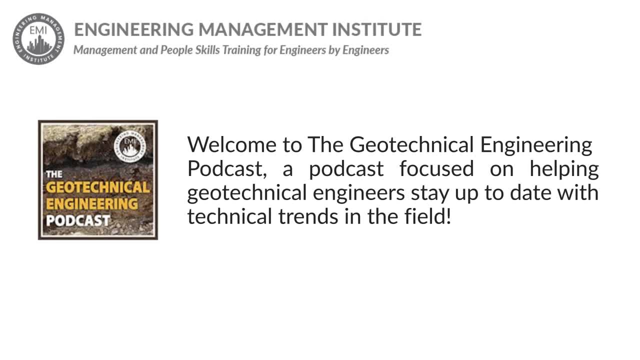 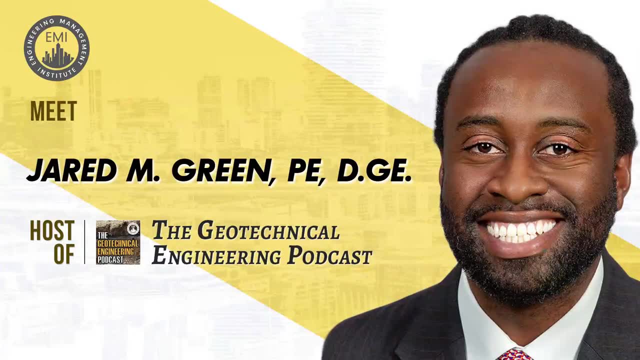 Hello and welcome to another episode of the Geotechnical Engineering Podcast, A podcast focused on helping geotechnical engineers stay up to date with technical trends in the field. I'm your host, Jared Green, and I've practiced as a geotechnical engineer for over 17 and a half. 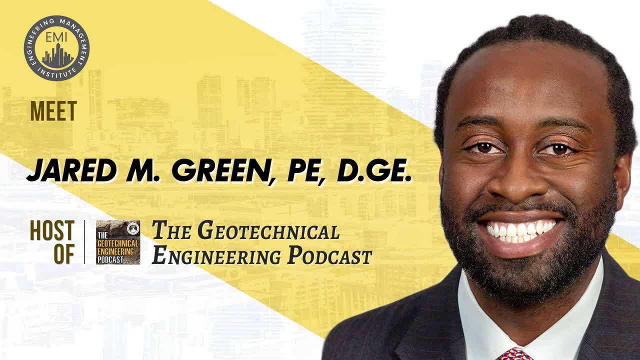 years. In addition to practicing engineering, I enjoy mentoring young engineers and first generation college students. I focus on helping to increase the number of pre-college students that are interested in STEAM majors and fields. STEAM is science, technology, engineering, art. 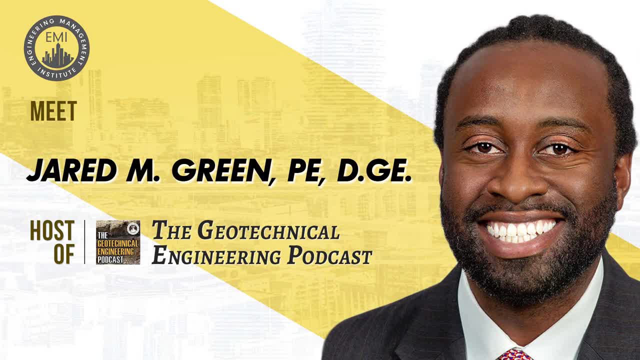 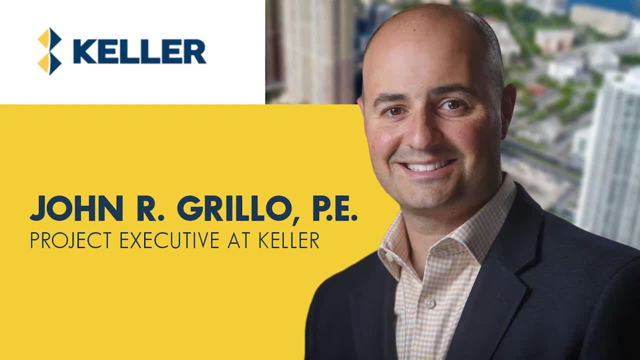 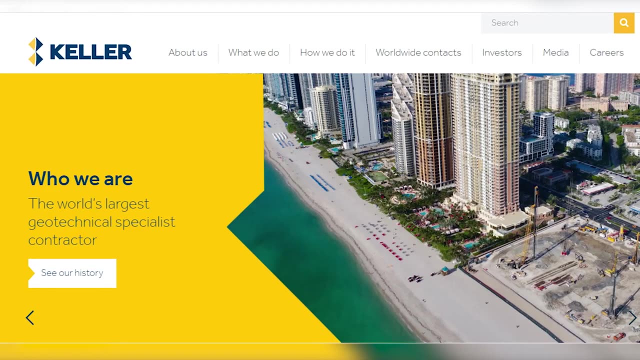 and mathematics. In this episode of the Geotechnical Engineering Podcast, which I may sometimes refer to as the Geopod, I'll be talking to John Grillo PE. Mr Grillo is a project executive at Keller North America Incorporated. He's been a member of the Keller team since 2011. 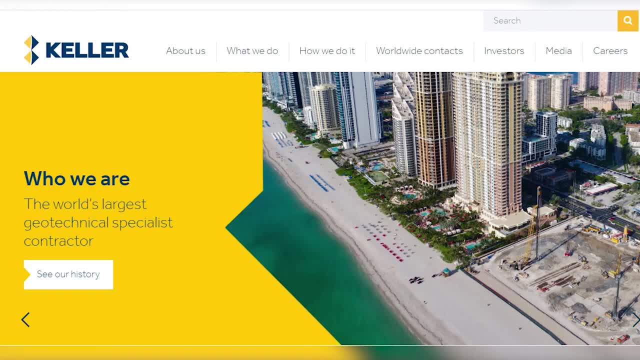 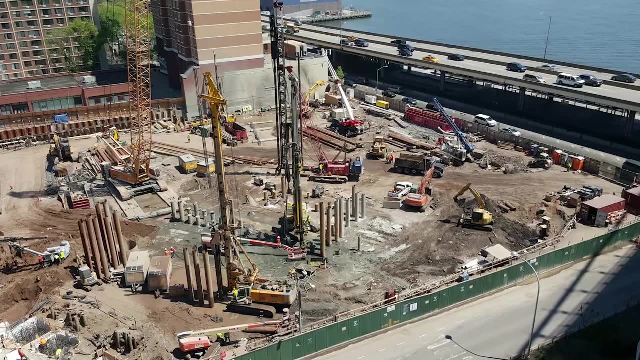 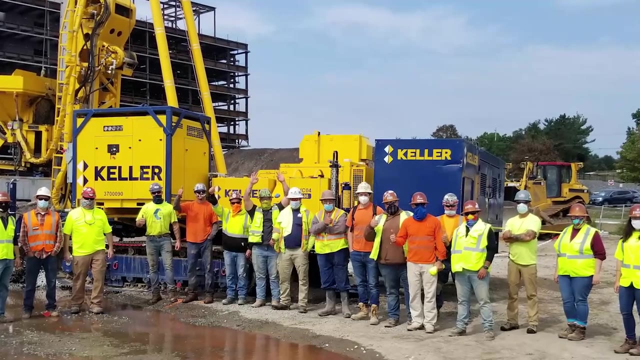 and has over 15 years of experience as a geotechnical engineer and specialty contractor. John is currently the ground improvement division manager for the Rockaway office. John has been involved with the design and construction of excavation support, underpinning, micropiles and macropiles, secant pile walls, auger cast piling, ground improvement. 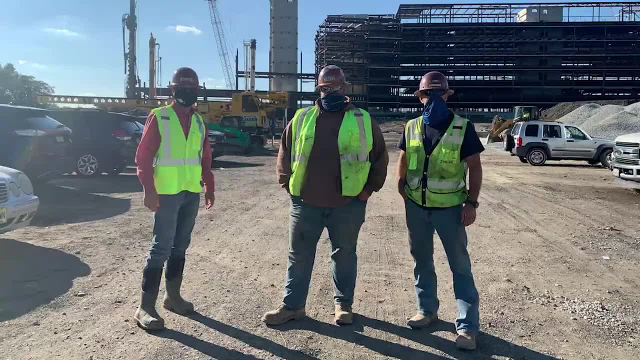 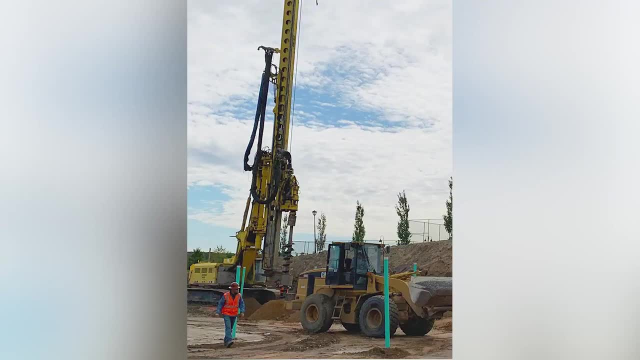 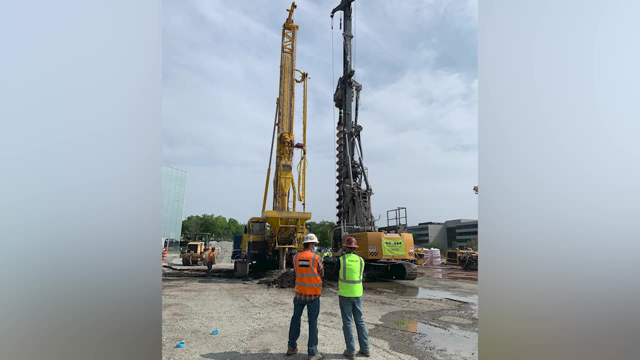 and driven piling projects, mostly in the private sector. He's also involved in the research and development of drilling techniques and the procurement of equipment and tooling to help keep Keller as an innovator and ahead of the competition. John is a licensed professional engineer in the state of New York and also in the state of New Jersey. He has a 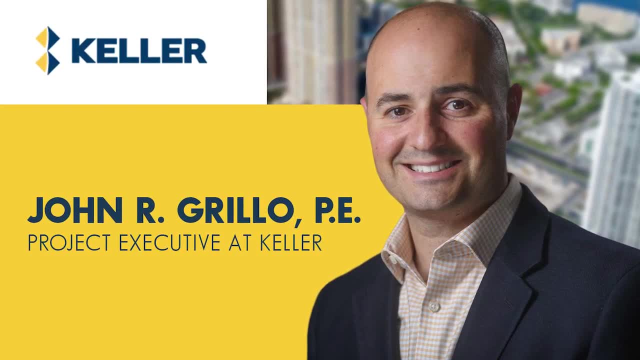 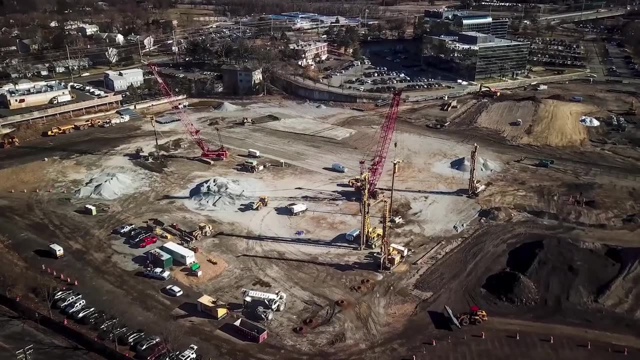 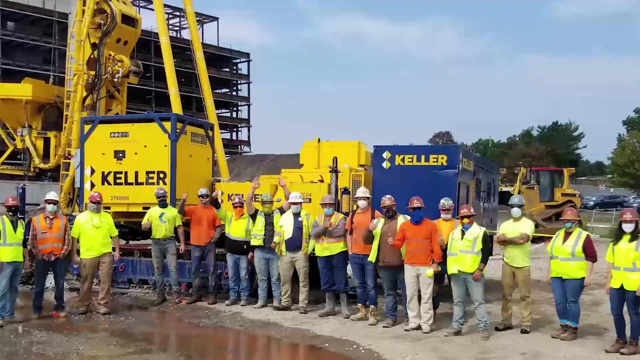 bachelor of science degree from Manhattan College and a master of engineering degree from Cornell University. Outside of Keller, John is currently the secretary of the board of directors for the ADSC Northeast chapter and is the past chairman of the ASCE Geo Institute of the MET section. 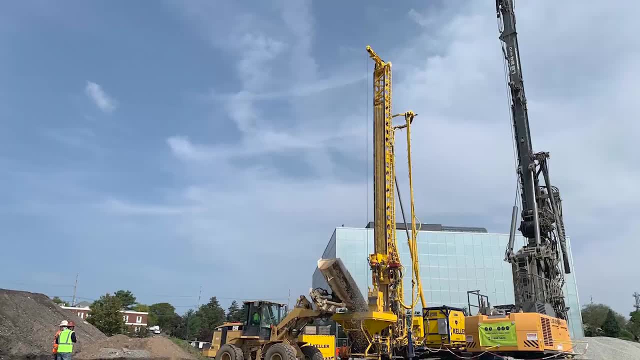 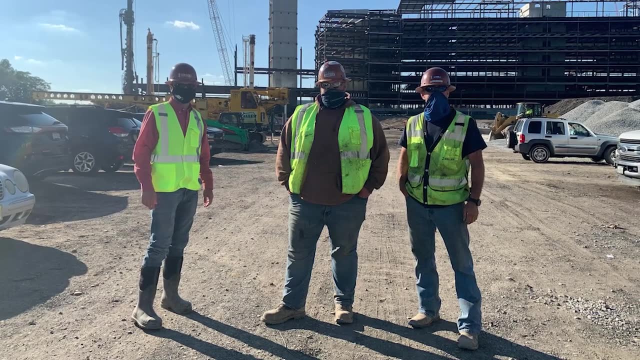 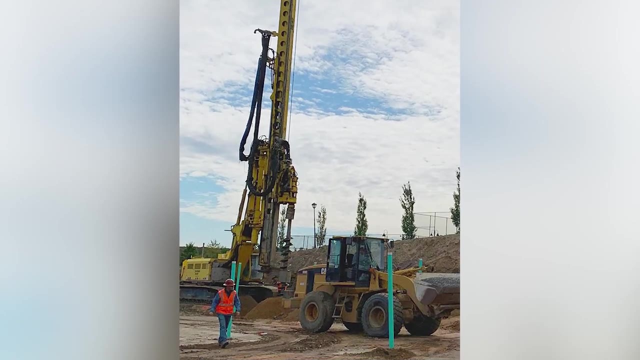 Very recently, just a few weeks ago, DNR Engineering News Record New York just listed their top young professionals, And these 20 under 40 include Mr John Grillo. And with that let's jump right into our conversation with John. 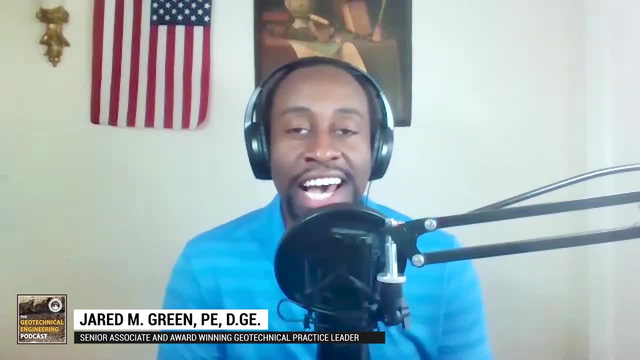 John, welcome to the Geotechnical Engineering Podcast. We're honored to have you. How are you feeling, man? I'm good. Thanks, Jared. Thanks for having me. I really appreciate the invite and I'm excited to be here. 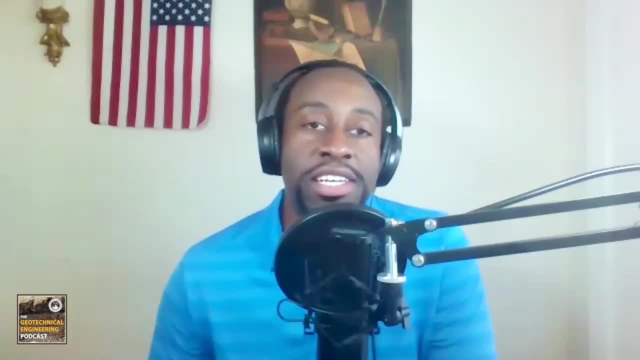 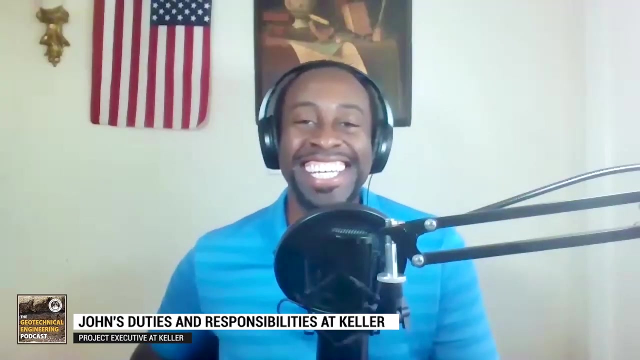 Excellent, Excellent. Well, if you could, in your own words, can you tell the listeners a little bit more about, let's say, your daily routine? Like, what does it look like working at Keller as John Grillo? So I do a little bit of everything. I'll make coffee in the morning, No, but for real, my job. 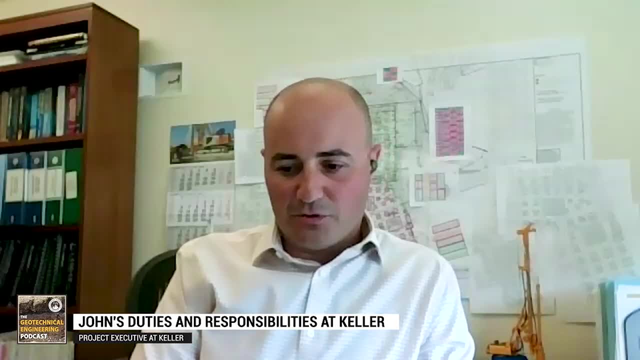 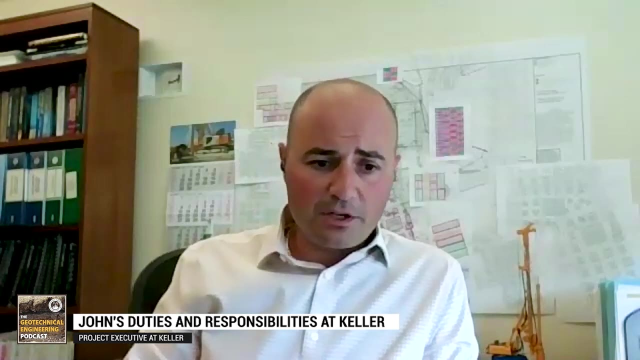 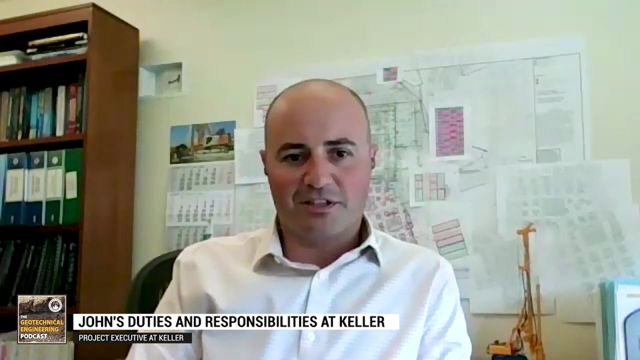 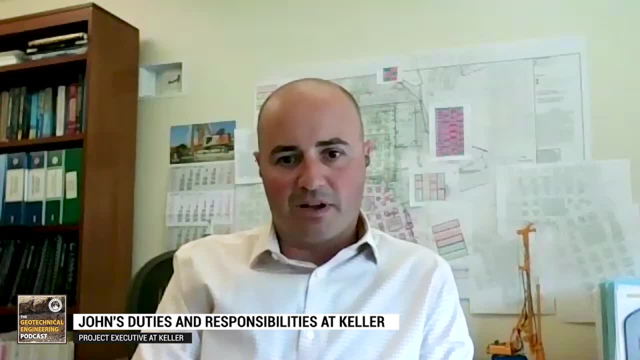 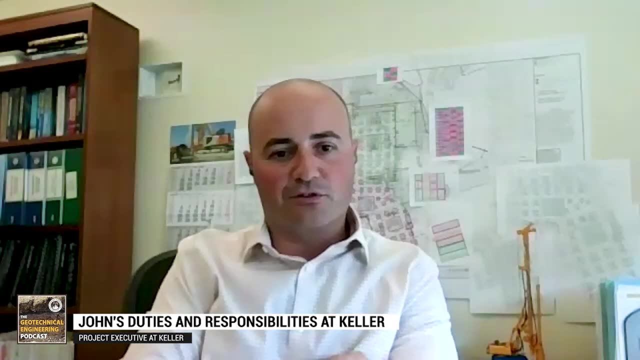 cradle to grave on jobs, Not as much being a soldier project manager. I used to be a bit more in a management role, now with in a management role now with with a group of project managers that that I work with to do get through the jobs. 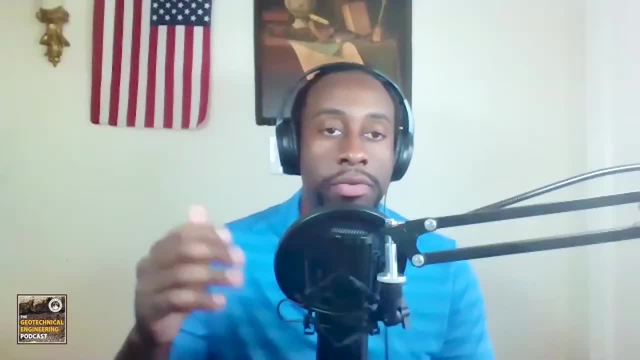 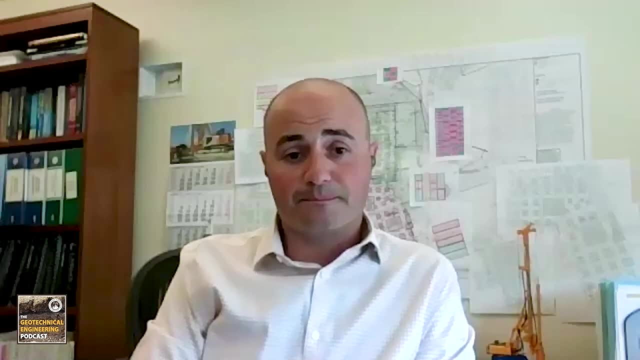 Got it, Got it. So it sounds like you're seeing from beginning to end, really in a lot of the back of house, as they would say, for for the whole division right for ground improvement, Yeah, Hmm, Ah, that's great, That's great. And I guess, if the ground improvement division manager, you know, and I think 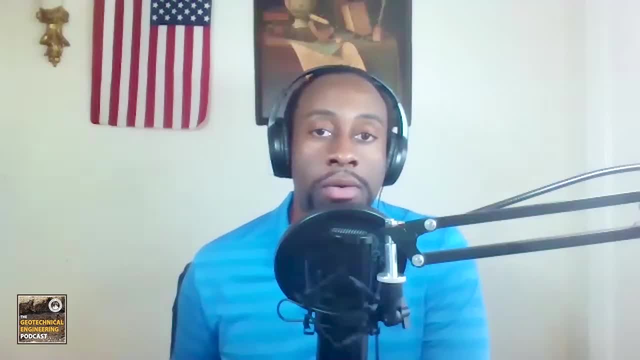 a ground improvement, or when I think of foundation design, one of the questions you know, before you just say we're going to have a deep foundation, is: what can we do with that soft ground? Can we improve it? Or if there are poor site fills, can we improve them? And that's really what your focus. 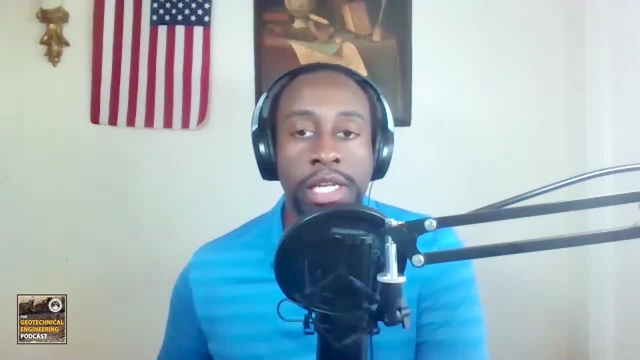 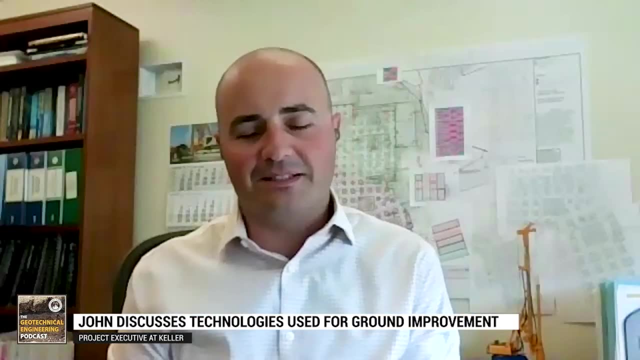 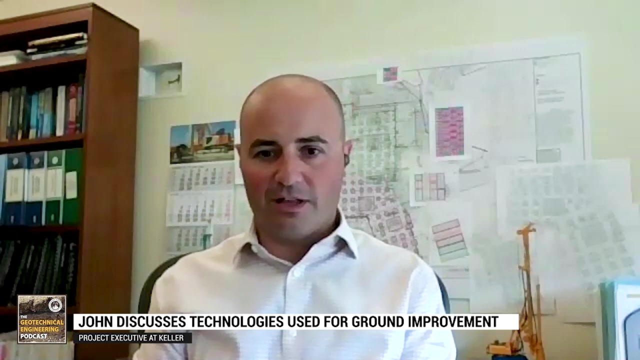 is. So I mean, can you tell us a little bit more about the improvement technologies that are out there, Like how do you actually improve the ground? Sure, So the main technologies that there's. there's two main technologies that we use for for mostly for building foundation and in a lot. 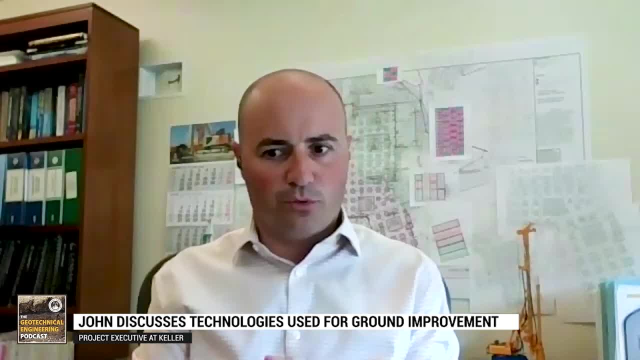 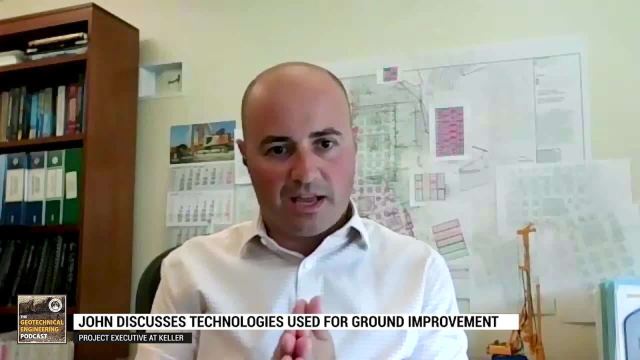 of like the intermediate structure, where it's not too heavy, where you would have to get something that's a deep foundation. Typically we do a lot of stone columns, aggregate piers and rigid inclusions. Those are two main techniques. I mean there's also, you know there's, there's all types. 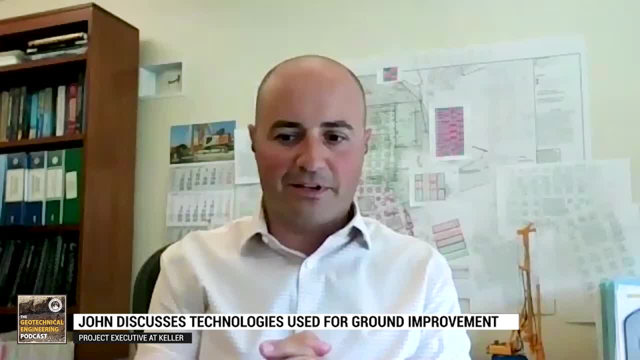 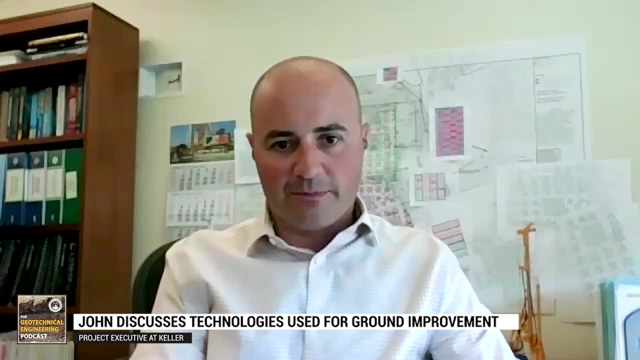 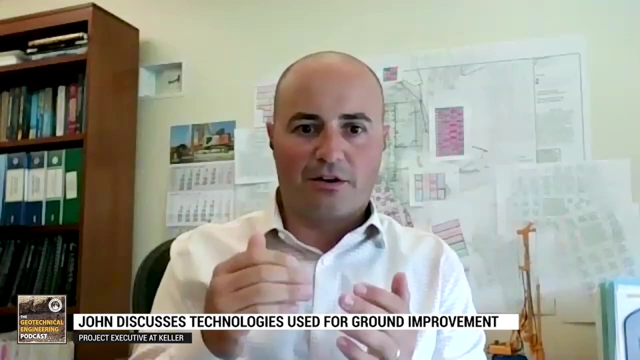 of grouting. grouting you can do for ground improvement as well- but mainly the the focus that I work on is typically aggregate piers and rigid inclusions, Because really I mean, there's there's buildings like logistics centers and you know the three to four story wood frame. 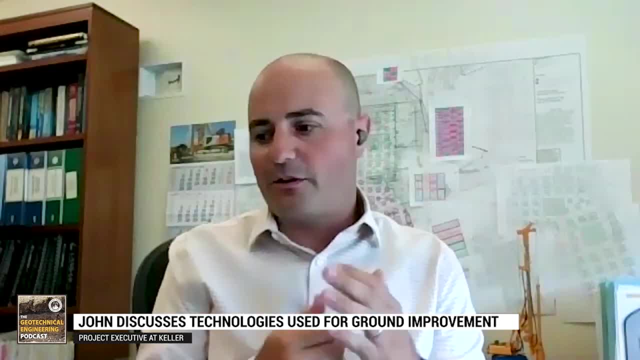 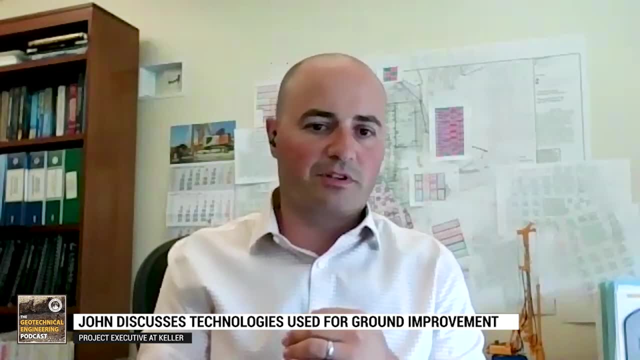 residentials that are going up all over the place and and they're really not too heavy, So when the ground just needs a little bit of help, that's where a ground improvement can can can save the owners and developers a fair amount of of money versus. 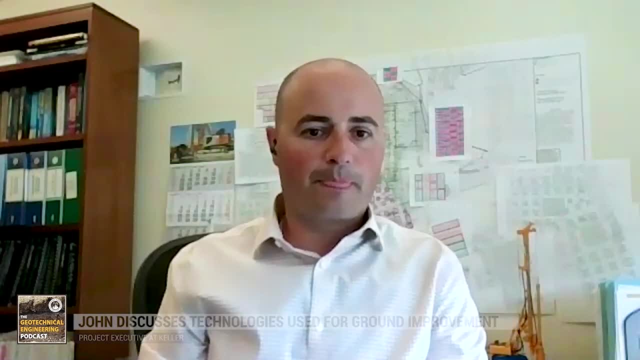 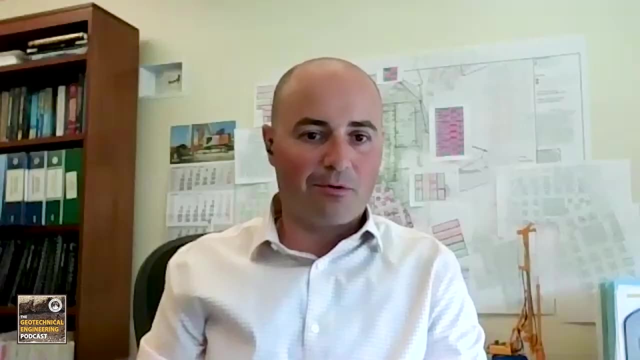 say, driving piles or drilling structural piles Makes sense, And I imagine for slabs as well. like you wouldn't want to pile, support a slab if you're sitting on a grade. Exactly Right, You'd have slab on grade over ground- improvement for sure. 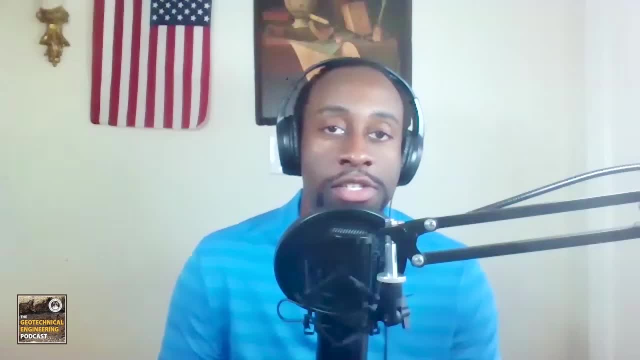 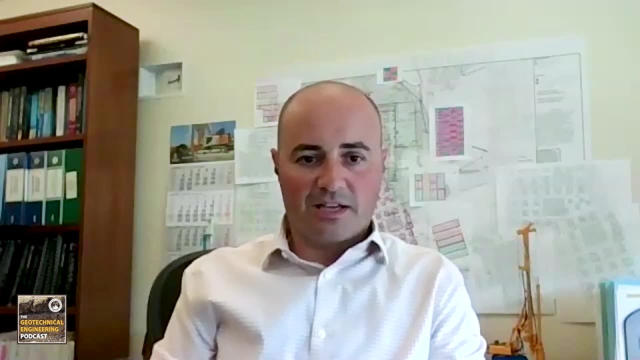 Okay, And can you break down those two different types, just for you know, for the listeners that haven't done any of this before? Sure For a structural slab, essentially as if you had a, the second floor of a building would be a. 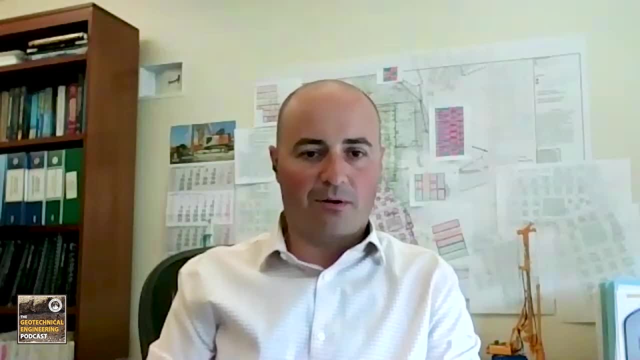 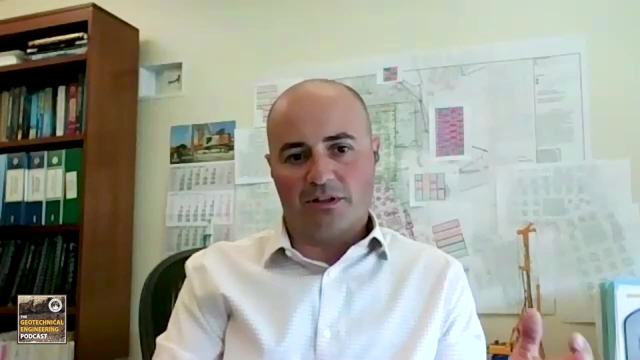 concrete slab. that would be a structural slab, Meaning you're not, you know, would count on any of the support from the soil below it. So you would install a structural deep foundation element, you know, at some type of grid similar to a columns. 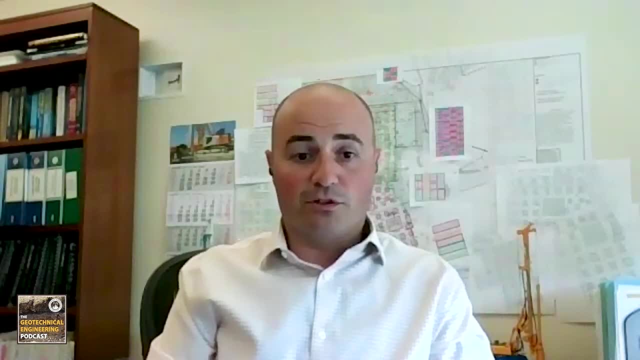 in a building to support that slab. If you're using ground improvement and using a slab on grade, you're counting on the ground to provide the support for that slab and to control settlement differential and total. But what you're doing is you're improving the ground to. 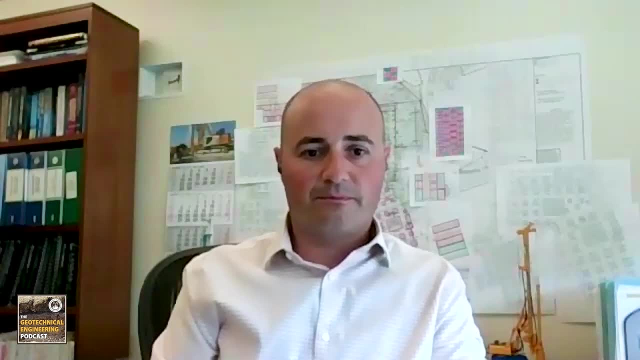 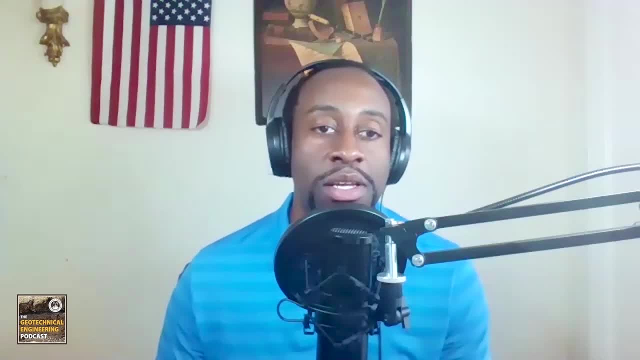 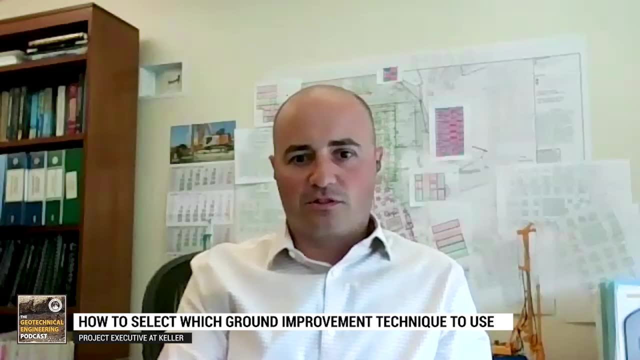 know which one's going to be appropriate for a job. Of course it depends, but you know what are you looking at to determine which way you'll go. So a lot of that starts at the beginning. I always joke around, like you know. I got you this big. 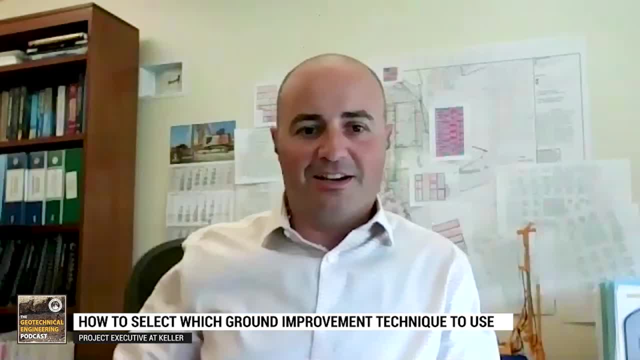 pile of stuff to do. And where do you begin? It's the beginning, So I kind of take it in a progression Like what's what's the least amount of work we can do And is that you know, you're. 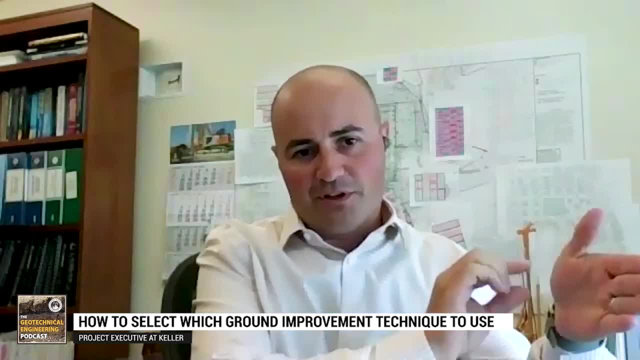 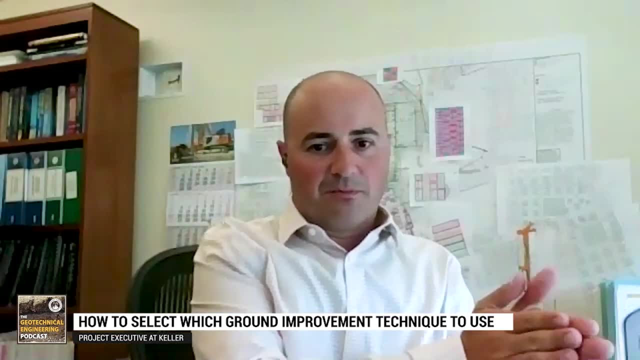 looking at, is that- and I don't mean at the least like not good enough. but you know you don't want to. I don't want to overscope a job and do too much work. So if we look at something similar, 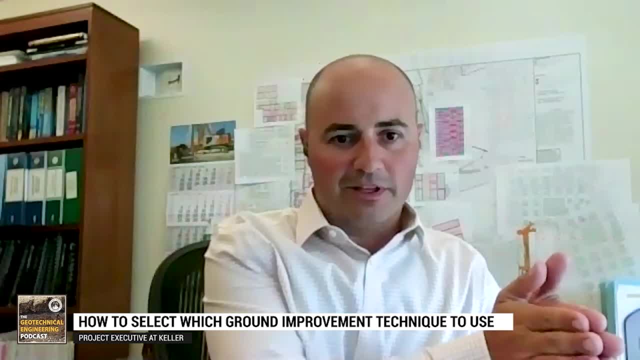 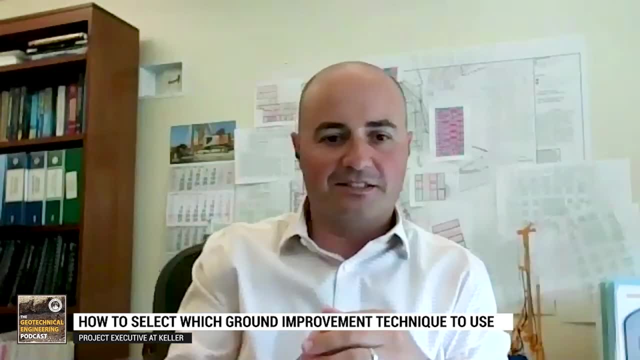 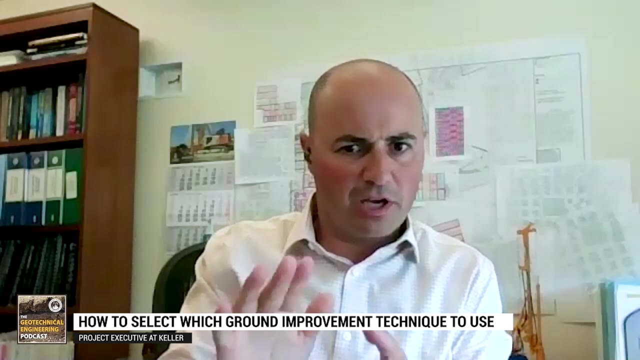 to like a compaction technique, like a rapid impact compaction. that would be like the least amount of work I can do on a job. Does that, does that fit the bill? Well, no, like. well then the next bucket is, say, aggregate piers, And that works really good. You know, typically up to about 40. 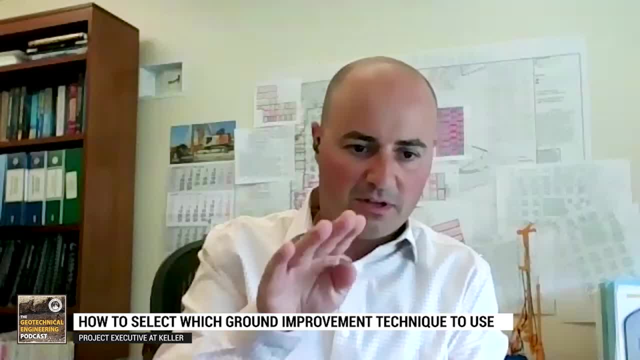 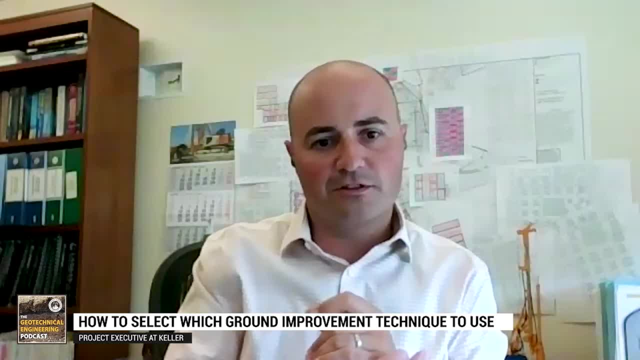 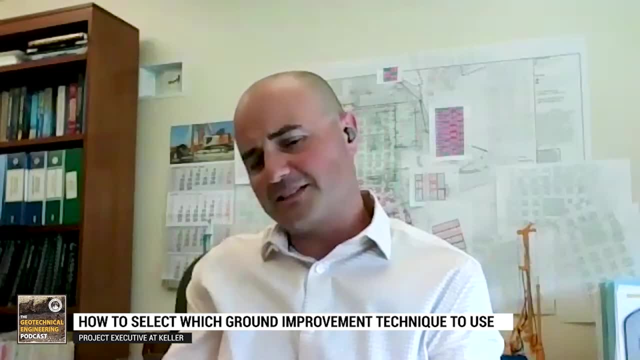 40 foot range where you don't have very thick, thick, soft layers. that is it. That's going to do excellent job, excellent job improving that ground. And then, if you have the next level up from there, would be the rigid inclusion which is going to give you a ability to bridge through. 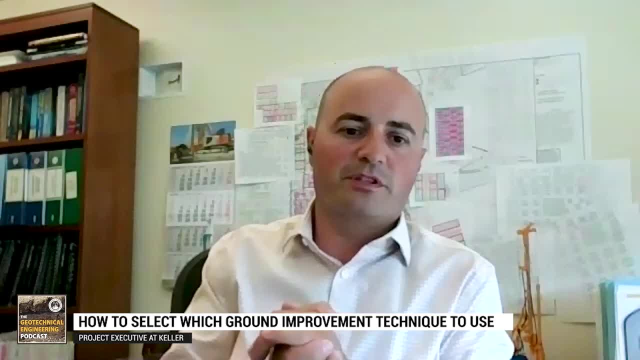 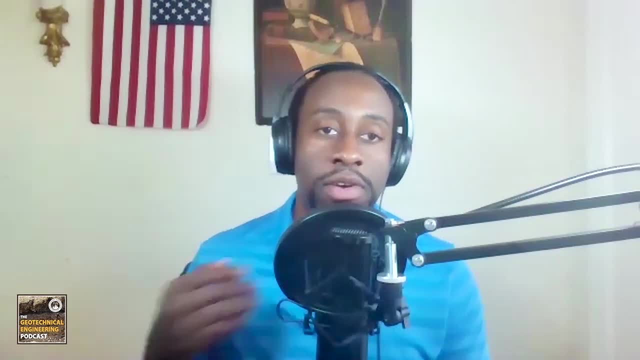 like deeper deposits of softer material, Excellent, Excellent. And you know I say before you were focusing in on ground improvement because I mean, when I knew you, I thought of you as a deep foundation guy. You know we're talking about drilled piles and 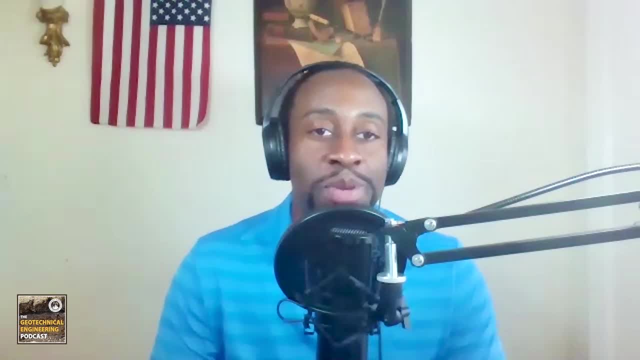 you know, caissons and things, that sort of mini piles, but you've made a transition from being, you know, focusing on deep foundations to more ground improvement. Can you tell us a little bit more about what that transition look like? or looks like, I mean, I don't know if you're still in it- 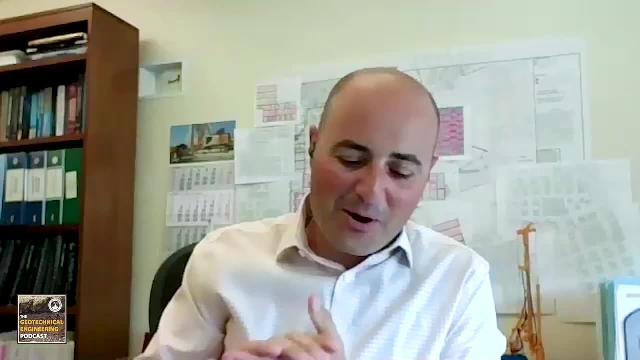 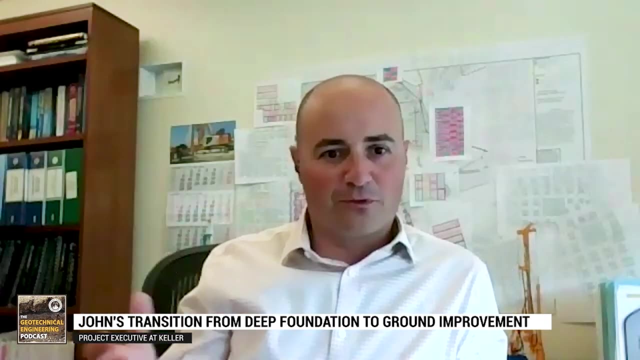 or you, or it's done, but can you walk us through that a little bit? No, I tell you that, that's. I tell the story a lot because it's it's been, um, it's been, uh, a wonderful journey so far. Nice, That's how I describe it. I can describe it. 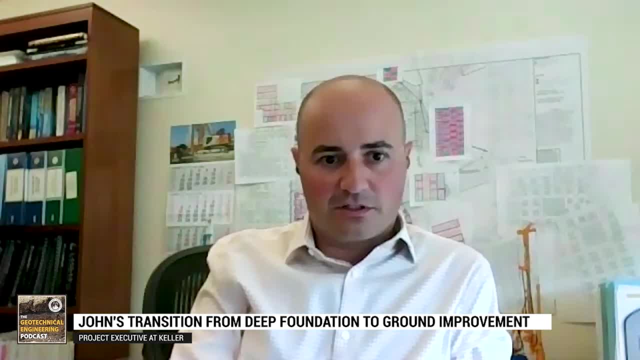 So, um, just about two years now. then this August, August 2020, is two years where, um you know, they said: Hey, like you just start looking at ground improvement here, Cause like that's a market where we're not doing a lot of in this area, but there there's market share. 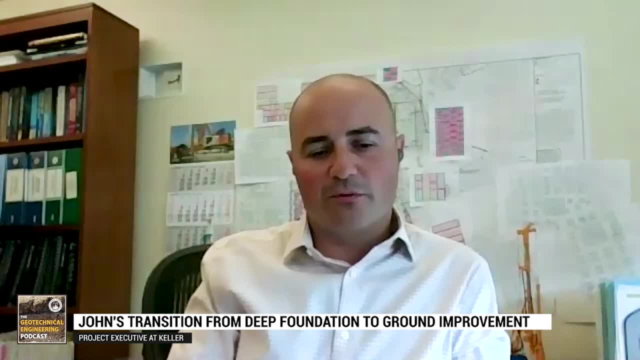 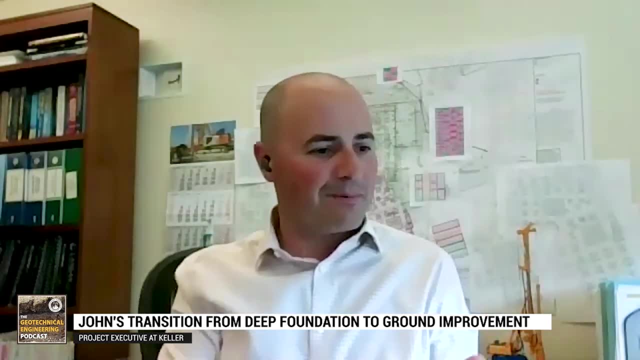 out there And you know, when we do this stuff, you know all over the country but not as much here. So can you, can you, let's, let's grow this business. And I was like, okay, challenge accepted, This is great, And you could do that about 50% of the 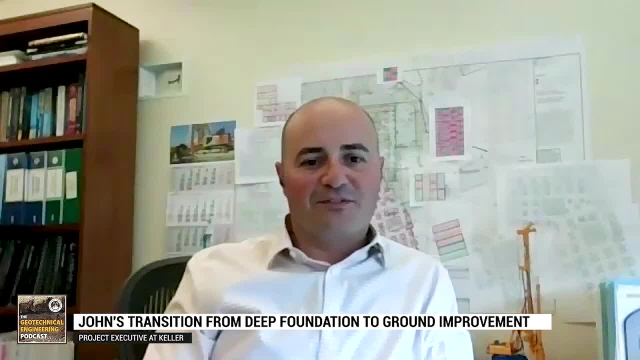 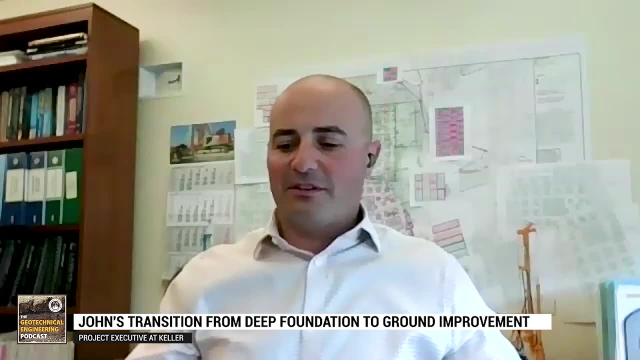 time You do your structural foundations and all that stuff, Um, you know, 50% of the time I'm like, yeah, no problem. So, um, I quickly found out that you know, like it's you gotta be all. 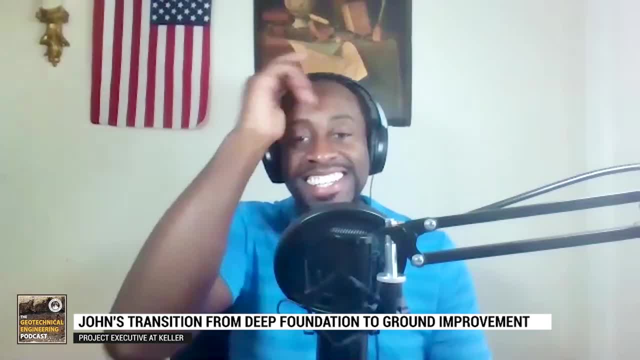 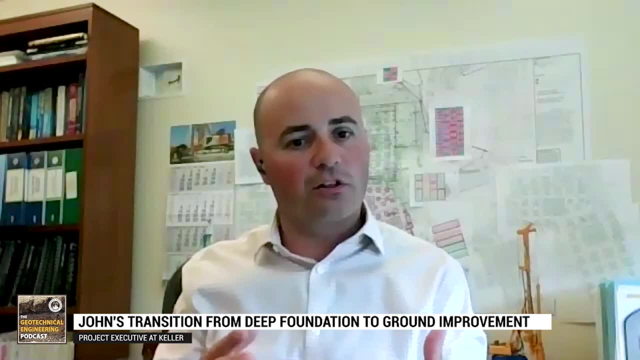 in: Yeah Right, I'm not going to do this. You know I can't be half pregnant on the on this stuff, You know. Um, I quickly found out like I had a really hard time juggling it, I had to like. 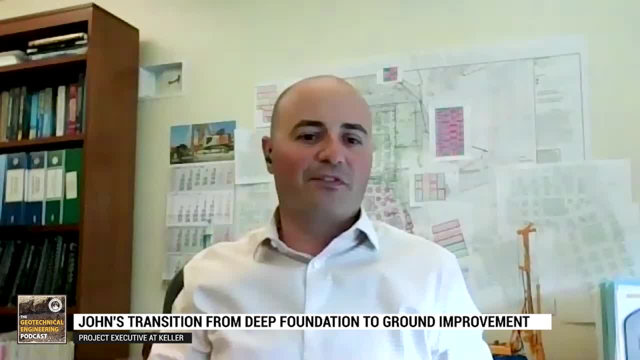 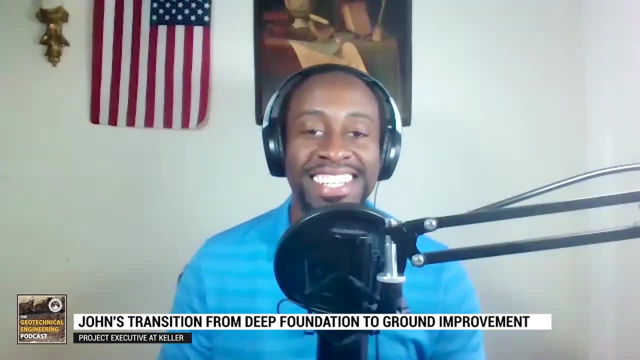 focus in and understand the ground improvement, because it was a lot different than what I was doing Cause previously. Oh, I'm going to drill a pile through that. I'm going to bypass that material. Now it's like wait, wait, hold on. Now I got to work with the material. Um, let me. 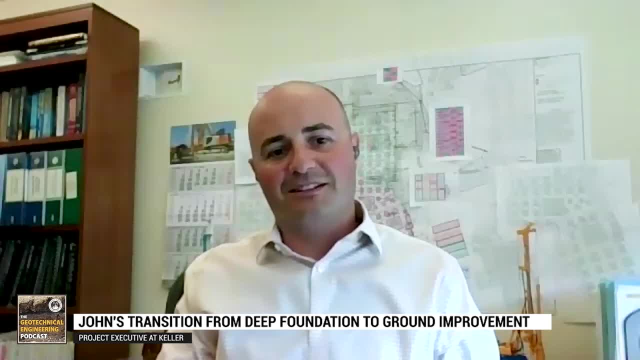 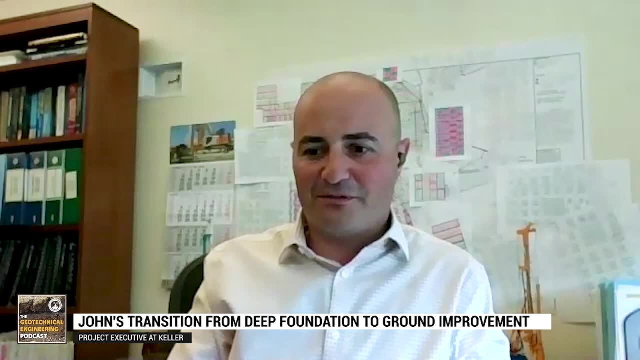 let me, let me kind of dust off some of those books and, you know, draw some more circles and and and go from there. Uh, so it was really good to kind of- you know it was, it was, it was. 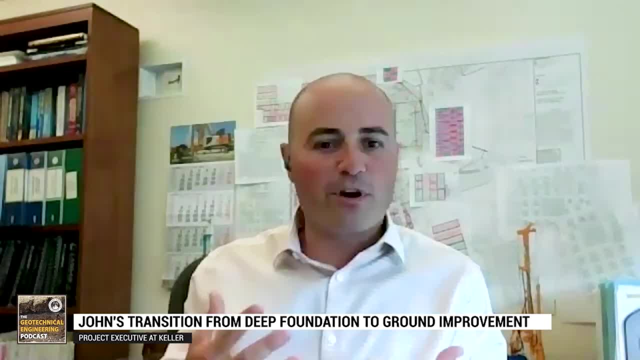 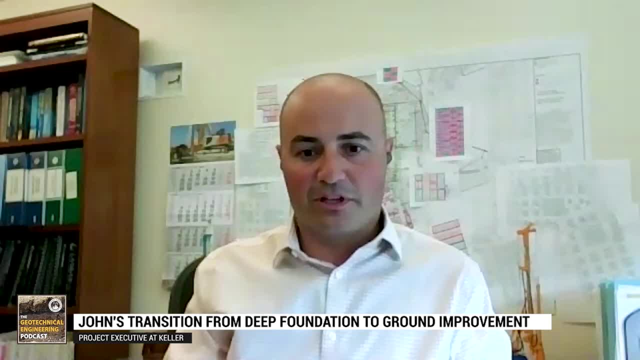 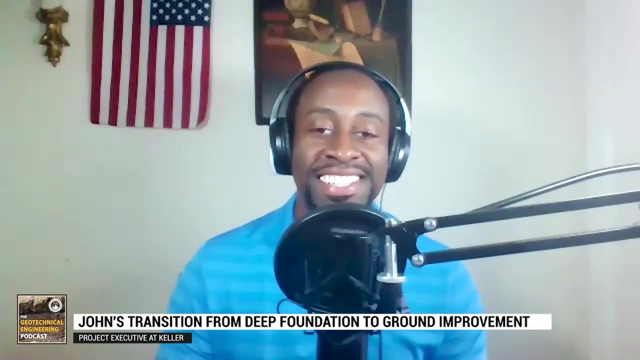 and those techniques that I haven't used in a while to, um, to really, uh, understand and learn the ground improvement. I really had immersed myself in it to understand and and get a feel for it. I mean, I, I, I, as you know, you, you are, you're a huge Ralph Peck fan, and um you, 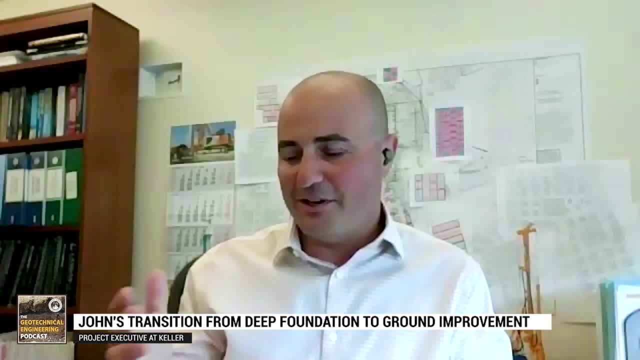 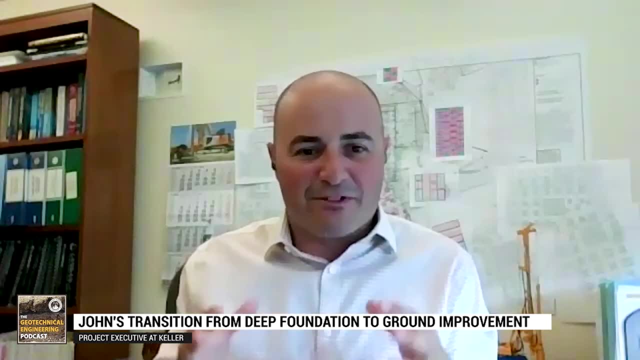 know, uh, you know the, the, the, the dear book about him, about judgment and geotechnical engineering. like I love judgment, you know. you know I love that Right, So I didn't have a spidey. 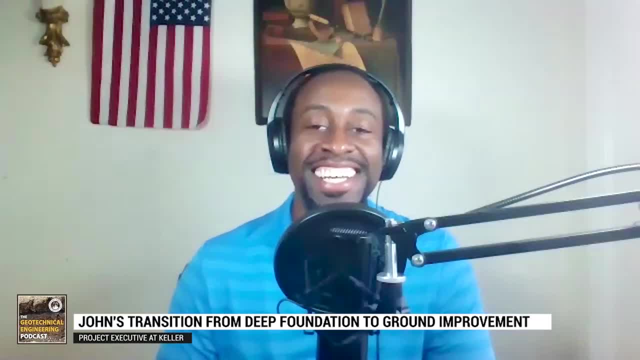 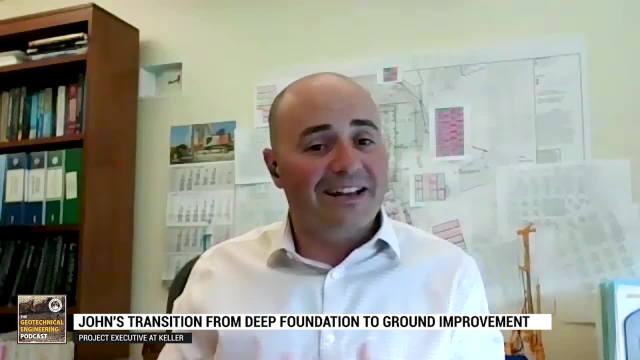 sense, Okay For ground improvement. Yeah, You know, I, I could look at a micropile and be like, ah, you know, it's full of PSI. right, I didn't have that, you know, And so I, I, I've, I've really. 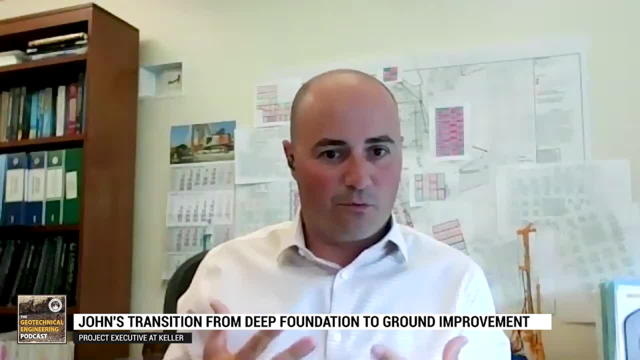 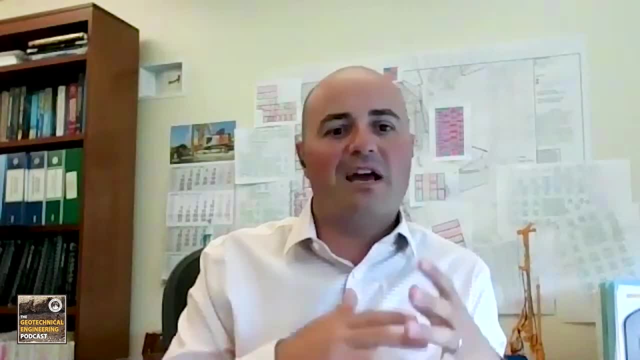 had to build up a, a sense of trust from what I was calculating or figuring out what it's going to be, and understanding and a feel for for how to use it and how to use it appropriately. Got it, Got it. And then every project that's completed is another data point, right. So? 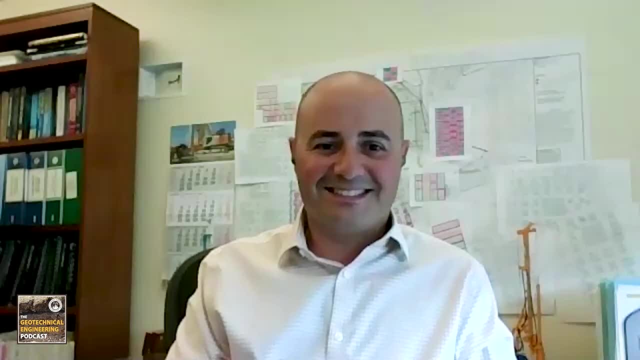 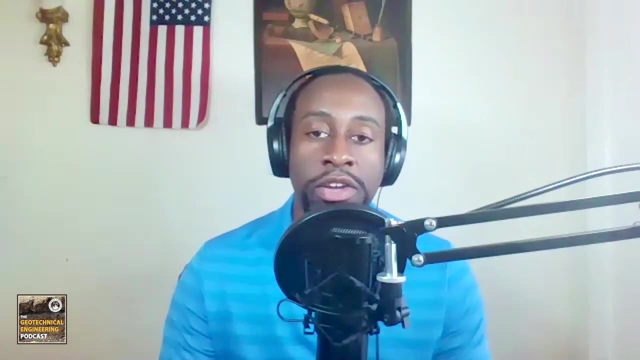 Oh for sure, Kind of calibrates the spidey sense in a in a in a way. Now, what are you doing as far as uh confirmation, Like, after you have improved the site, are you going back and uh doing CPTs? 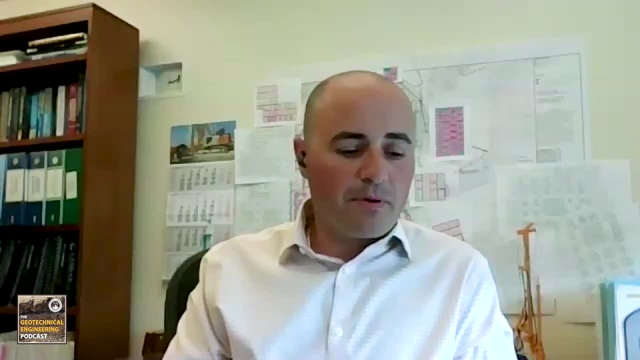 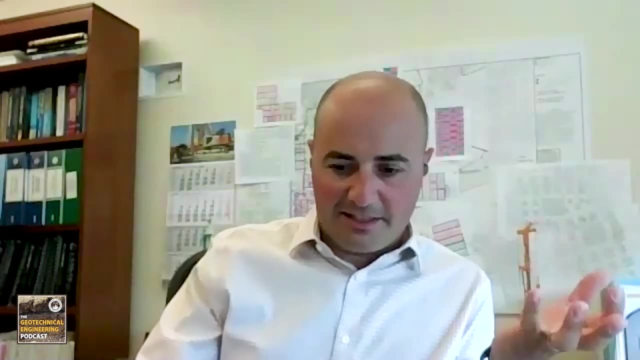 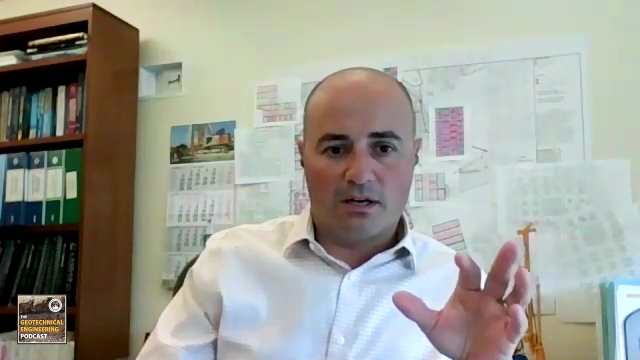 or borings to improve or So, depending on the project requirements. uh, typical structural support job or structural foundation that's. that's not dealing with things like liquefaction or uh, or or things like in that nature. Um, uh. 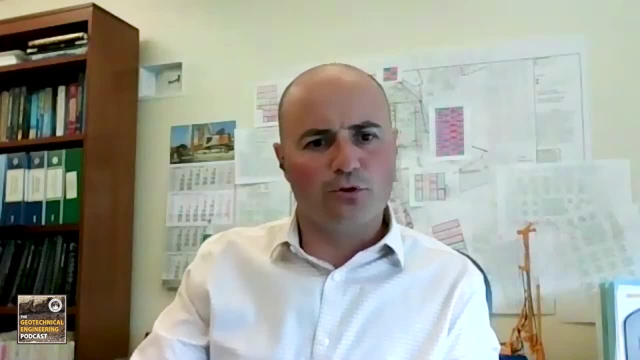 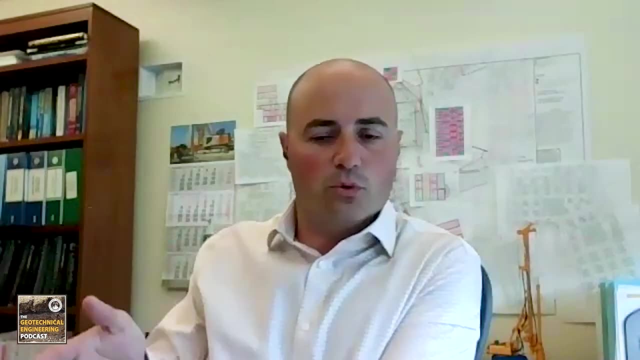 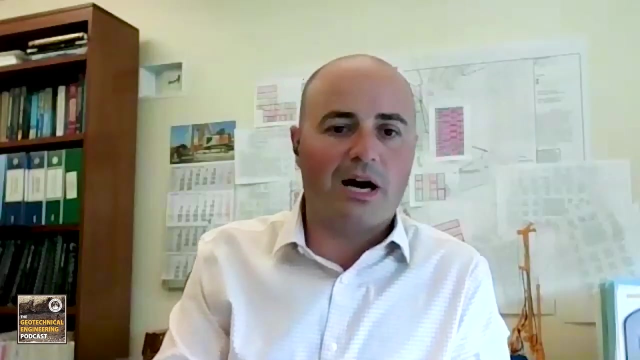 I think uh a uh. aggregate peer. we'll do a modules test on confirm the design, stiffness of the peer. We had assumed the design. we're doing a single element load test on a rigid inclusion Um. similar verification tests you would use in a, in a, in a structural pile Um, and as far as 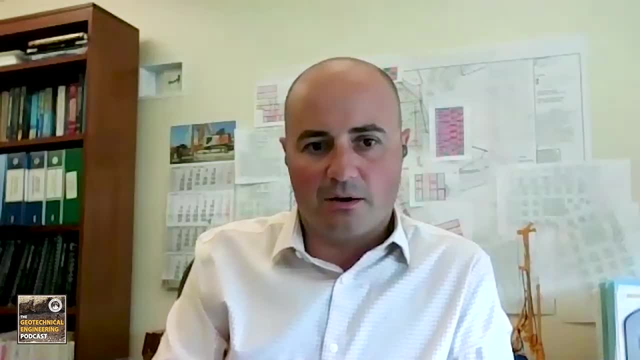 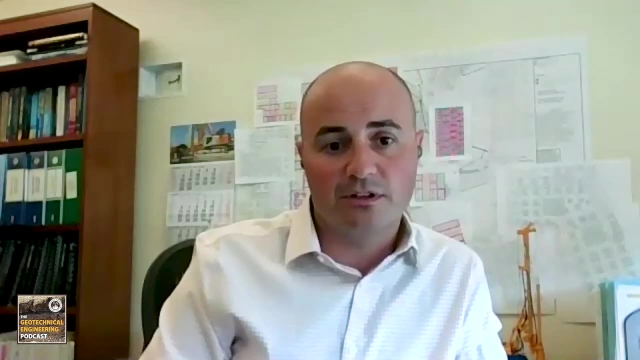 um that, like you mentioned that the post CPT or SBT, um, we've done some work um for uh, for kind of proven, it also doubled his lip of facsimil behöver. So doing that we've gone. 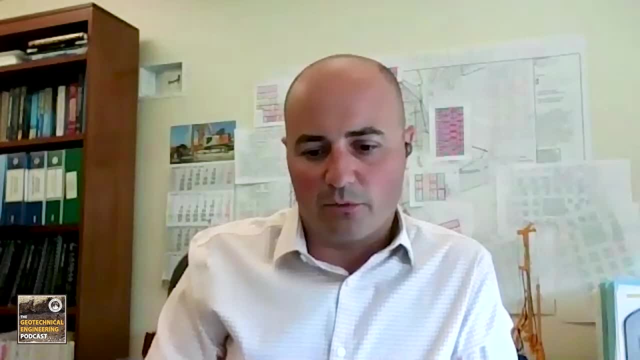 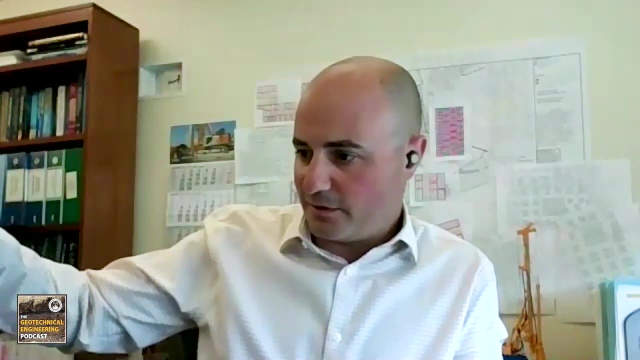 back and we've pushed cones, um, you know, and we've done them readily, from, say, an aggregate peer, you know, away from the center, for you know how much you know, get the furthest point away, and you know, and is that good? And as you get closer, 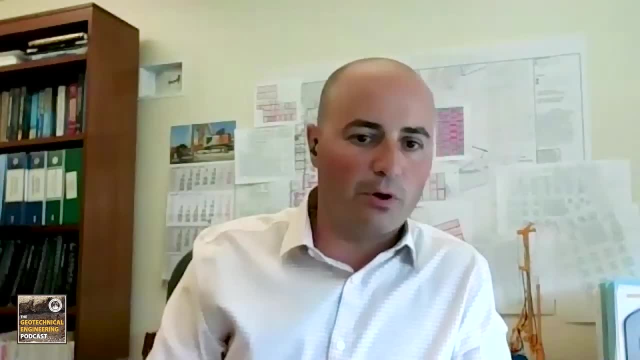 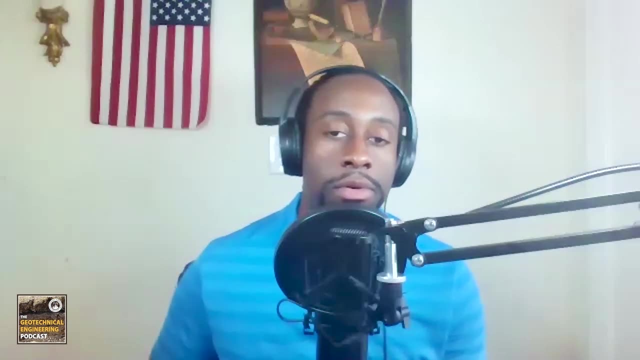 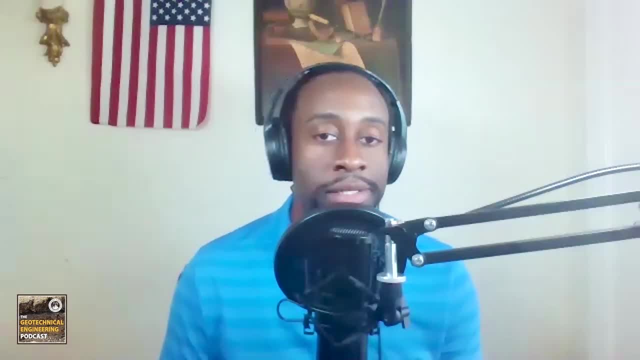 end Yes, On the− Audience Grounds. Christian nutrient level». what you would need in order to bid on a job? boring CPTs, specific lab tests. I mean what I imagine. more is better than less, but what's on your wishlist? 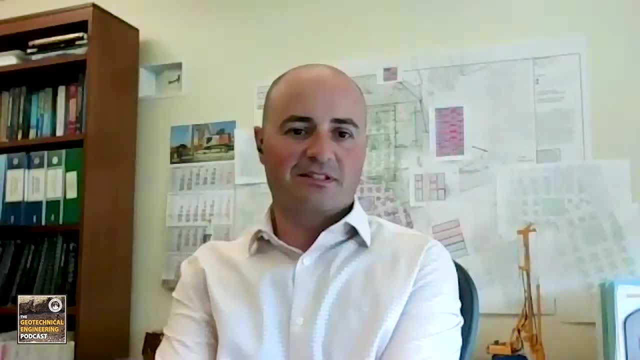 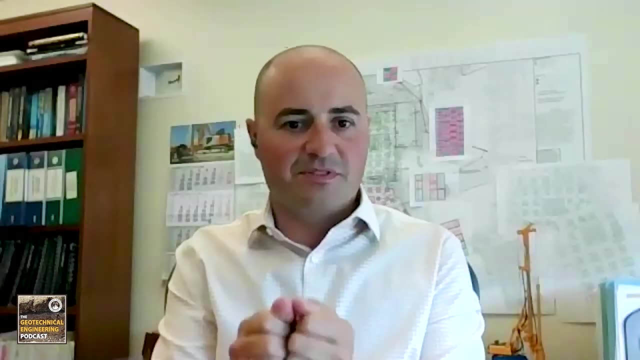 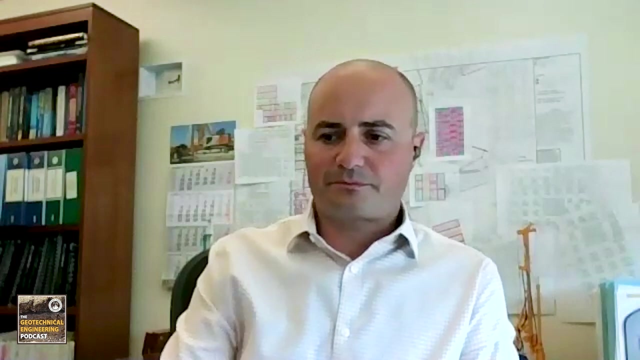 Definitely SPTs and CPTs. you know the SPTs, to physically touch it and classify it and get some, get some sieves and some limits. you know consolidation data is great and the CPTs are valuable because it's continuous information. 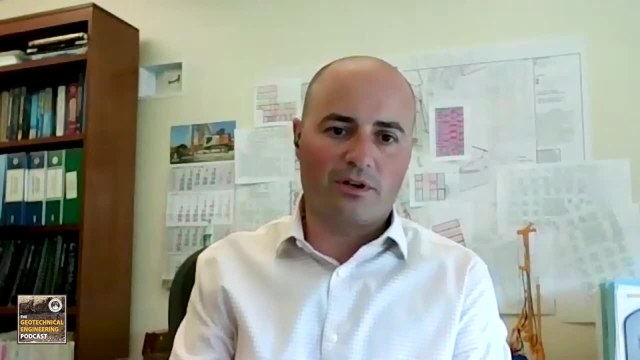 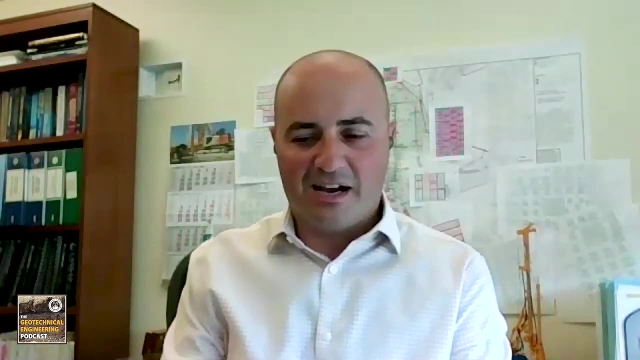 You're getting. you're getting a whole bunch of data points and you have a whole, a whole lot of correlation data you can grab from those points. I'm- I'm personally I'm not the biggest. I get a little fuzzy when you're over low with N values. 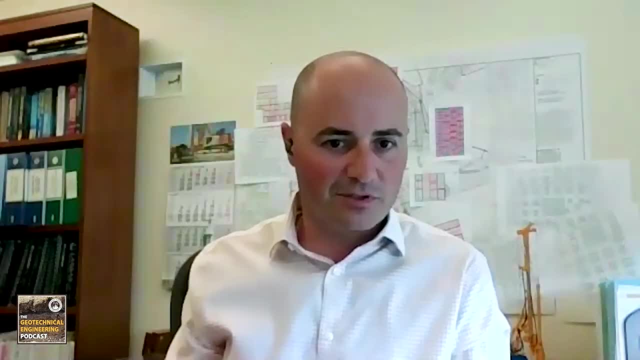 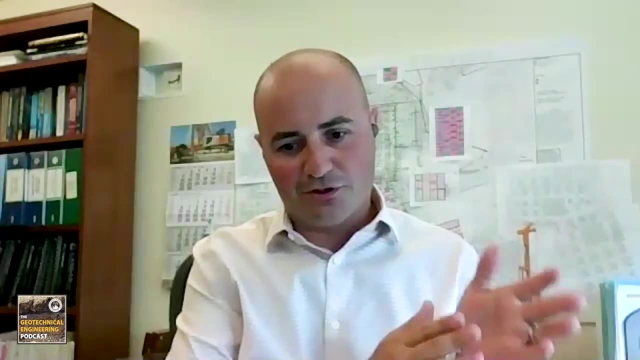 And I feel like you can, you can seek for clearly with the CPTs personally, Yeah, You know, on some of those data, because if you're really getting to the weeds and you want to correct some N values, you're going to. 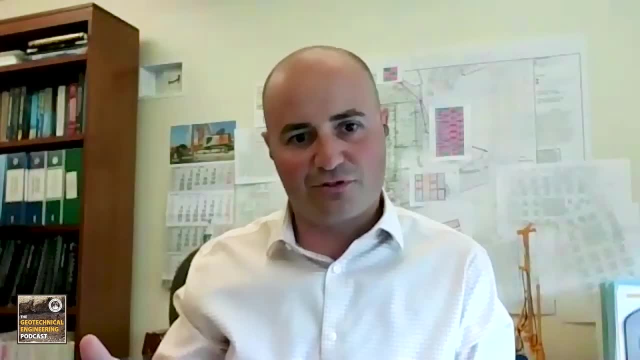 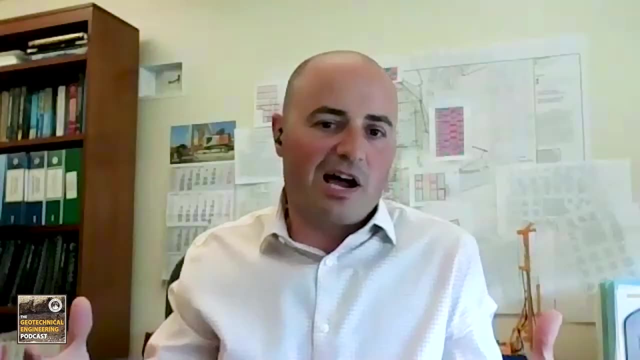 you can keep going down the rabbit hole. And so it's the CPTs kind of straighten you out a bit, Kind of go from there, And I mean the scale of the job will tell you the scale of how much more testing we can. 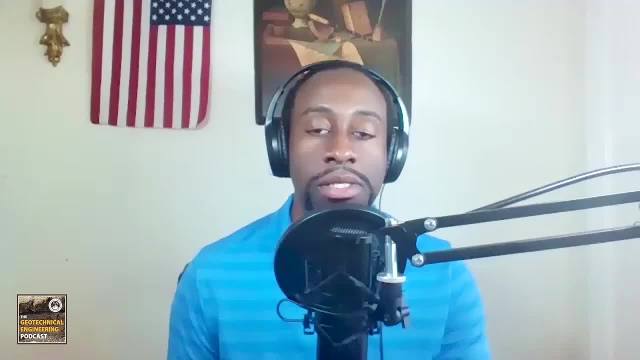 typically ask for and get you know Makes sense, Makes sense. And do you find yourself doing more work within, say, uncontrolled fill that was present at the site? Or are you more in native material? That's just, that's just soft. 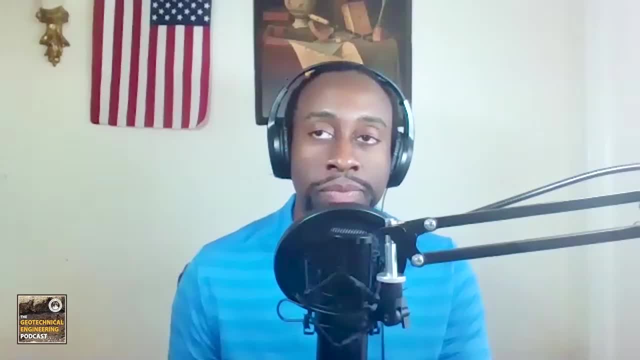 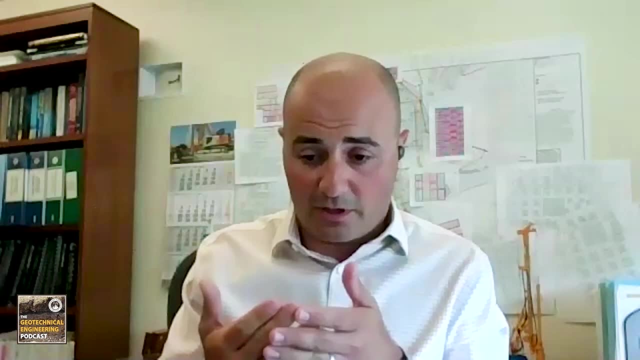 I'd say it's a good mix of both. Okay, Got it. I did some jobs where there was a concern, where there was a you know, uncontrolled fill, And so essentially the cause: the sand below it was in great shape. 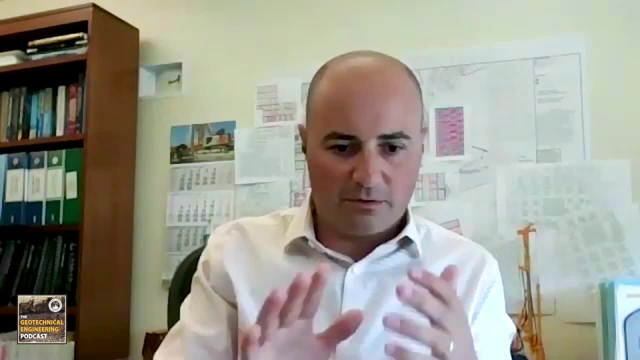 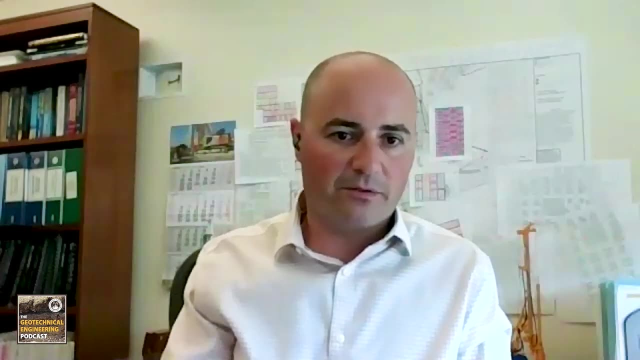 So essentially our aggregate peer system- kind of that job I'm thinking about- was 10 feet on center. We did 30 inch diameter peers 10 feet on center And at that point we had proofed out the the, the upper fill layer, and is very comfortable with the way it would behave at. 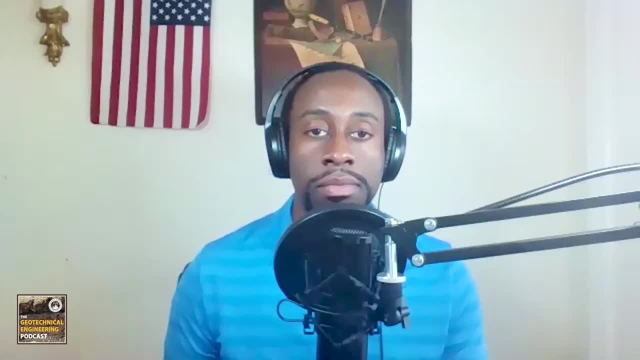 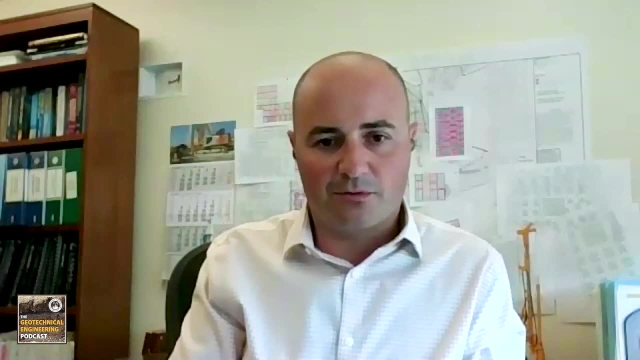 that point. So got it, Got it, And you know, and the plans behind me were for a for another job we did in North Jersey And and that was actually a lipofiber project And that was that was deeper aggregate peers in all native material. 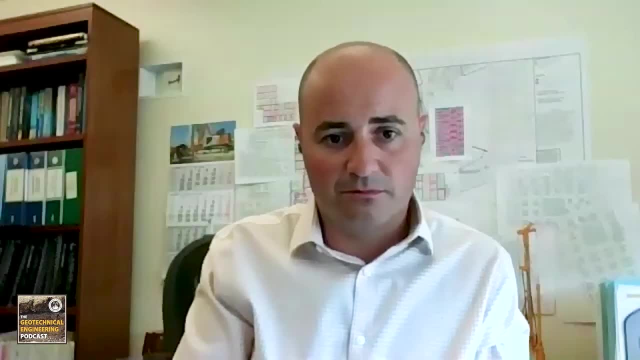 Oh wow, We didn't have any felt. We only had like two feet of fill at the top. That was. you know, it was all loose sands. You're into it at that point? Excellent, Excellent And from what I know of you, 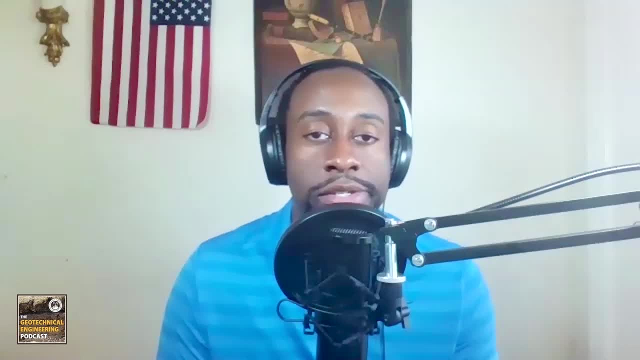 you. you've always tried to be on the cutting edge when it comes to research and development of drilling techniques in particular. But what are some of the latest techniques you've been implementing or hope to implement in the future? And, of course, you don't have to give any trade secrets. 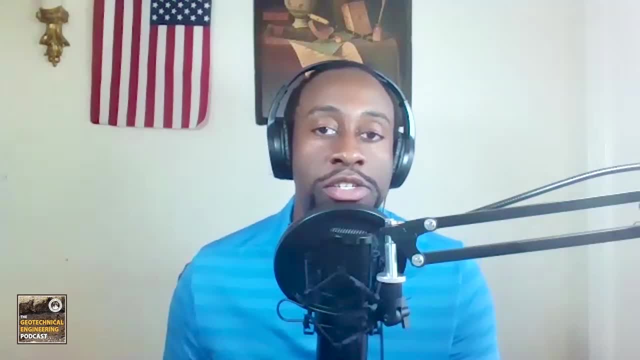 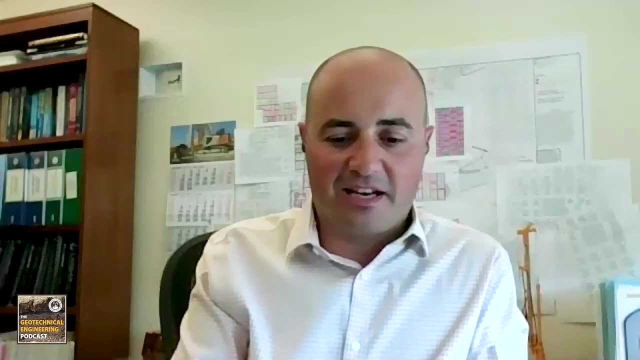 but you know, if there's something that some of our younger listeners, younger geotechnical listeners, may not have heard about, that you feel comfortable sharing, Well, yeah, I mean one, one technique that I that I spoke to you about a while ago is when. 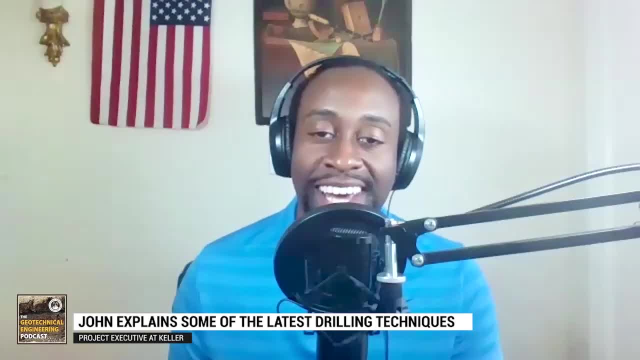 when we brought KCFA technology over here. Yeah, That was, that was the. I fought hard to bring that here and use it And it's been very effective And that was always. that's still a great technology and when the right spot. 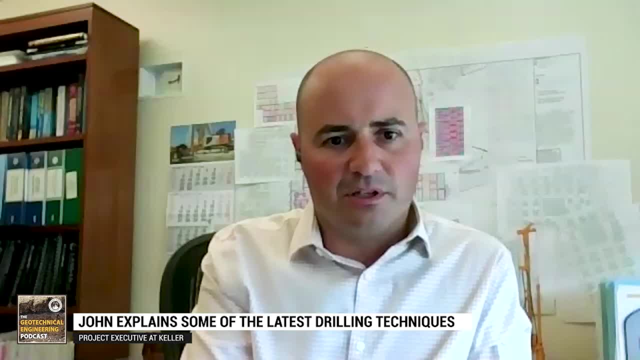 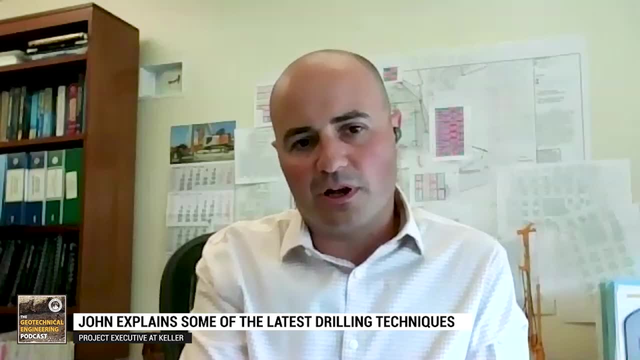 it's definitely the right technique. But, as of late I've been doing more work with. you know, installation of stone columns. you know, do you pre-drill, do you not pre-drill? How much energy does the vibrator have? 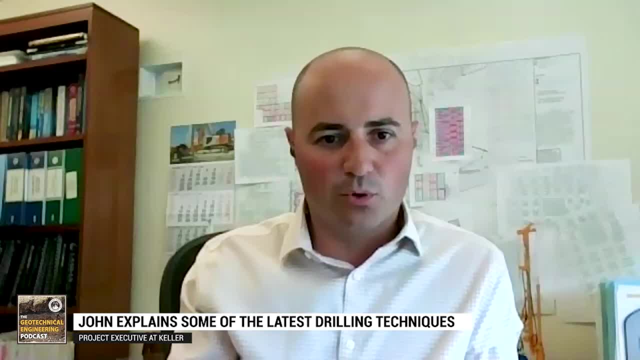 How big can you build stone? And on the original inclusion side it's been the tooling. you know heavy R and D focus in the tooling. What if we? what if we change the cutter head around? And you know. 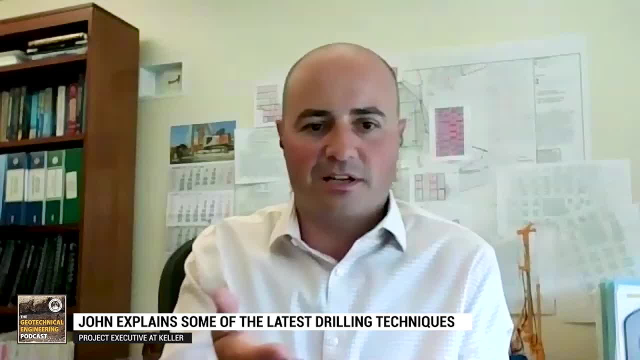 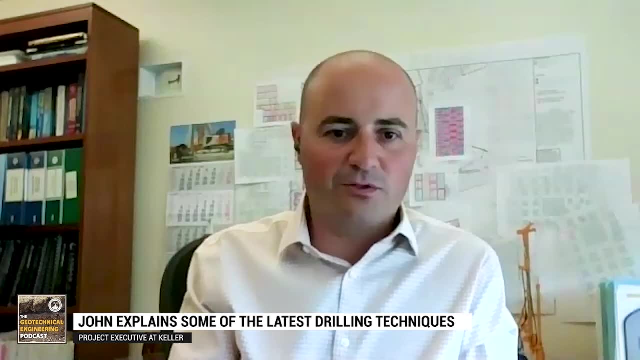 what about the grout orifice in the side? How big is that? It's a bottom discharge, a side discharge? What size drill rods? There's all sorts of different variables that, um, you know you try and tweak not too much at once. 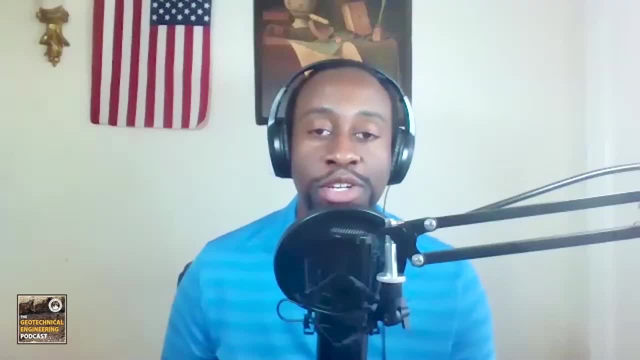 You can see what your control is. Got it, Got it, Got it. And how does that work? You go to the shop and you say I want to change this element right here, And then they change it and they test it and they get back to you. 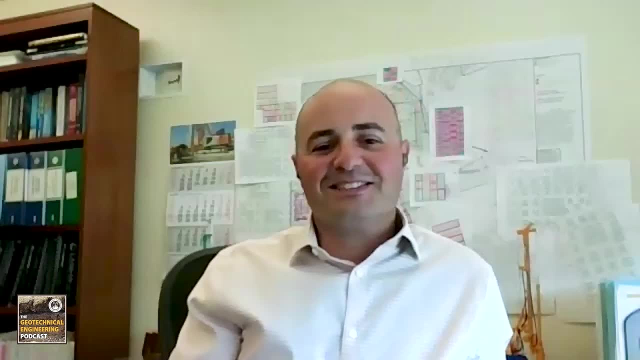 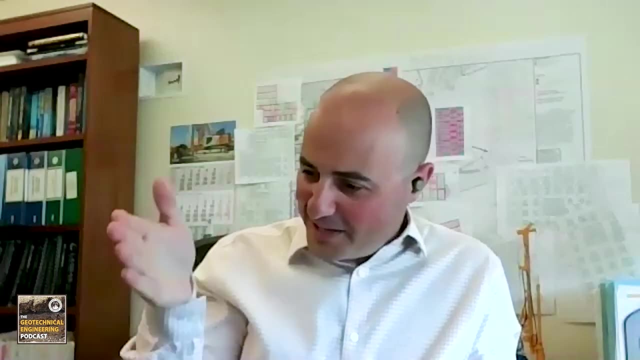 Like: how does that? what does that process look like? Well, you know, some of that stuff comes down to necessity. Sometimes, uh, you get, if you get a job and the tool comes, it's really worn on this one side of the school is really worn. 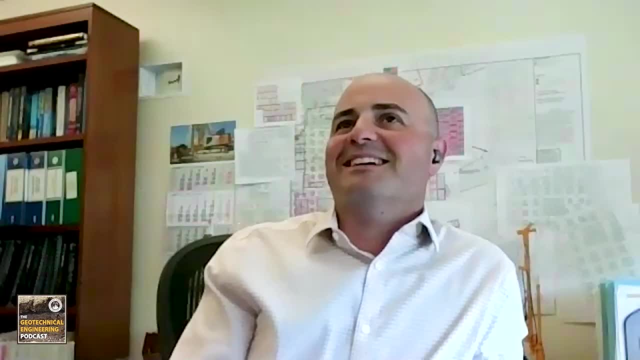 I'm like, Oh, maybe turn the tooth out a little bit and see what you know, see what happens. Okay, Um, you know all sorts of different. you know Frankenstein tools that you end up making and like. 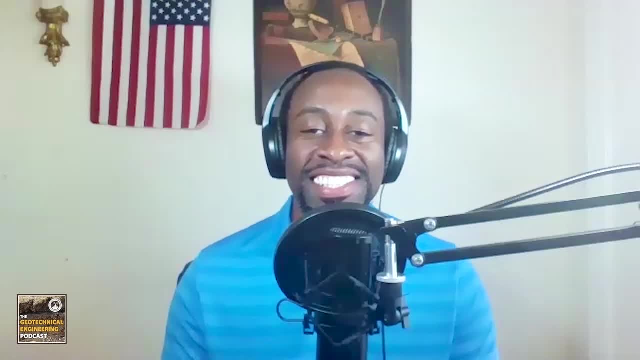 Oh, that one worked, We got to use that one again. Or, um, you know, and like, those paths kind of run parallel with, you know, some of the equipment manufacturers, that things that they're making, Um, and they're like. 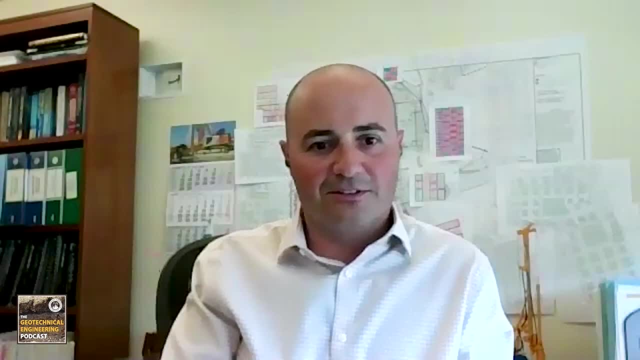 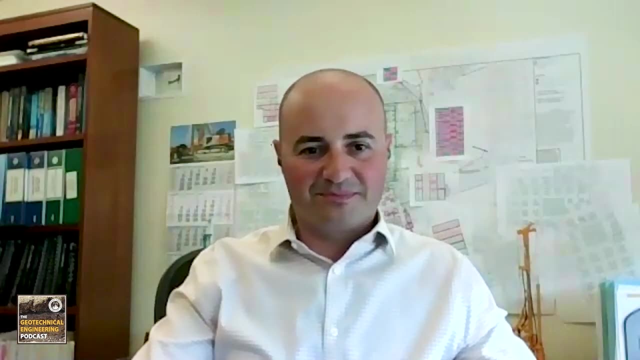 Hey, I got this new thing And I'm like, Oh you know, let me put this in this together. And you know, it's um, it's exciting. I mean, that's just I, the stuff that kind of gets me excited. 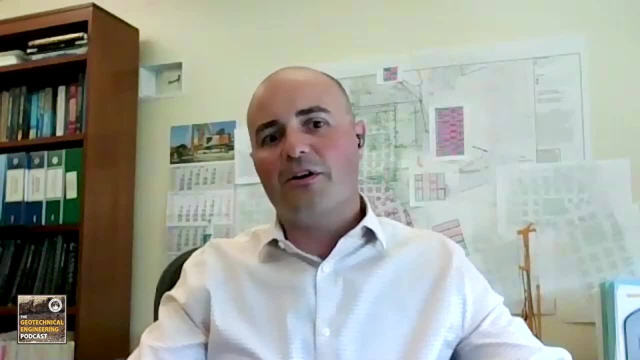 you know, excited. The tooling is definitely something that's always like, you know, Oh, and it's just there's a better way, I know there's a better way, you know. Yeah, Yeah, Yeah, I remember when you. 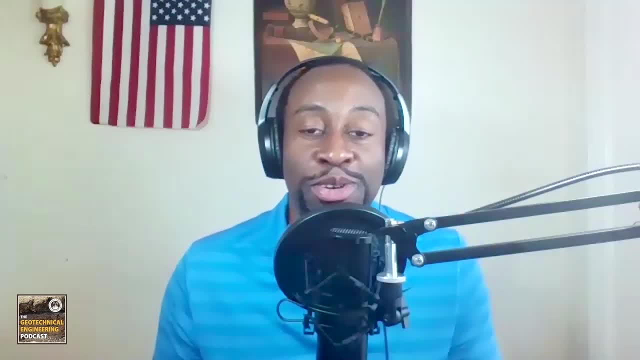 um, you know, I remember when you started your career- you really you know you're in consulting And when you made that transition over to working for a contract you really used to talk to me a lot about you know. 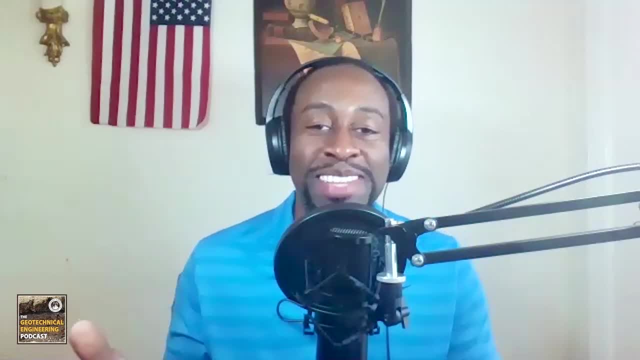 well, think about how it goes together, right, It's like you can't just spec something. I think about how it goes together and how it's actually works, So that's pretty cool. Like I think you had to go to drilling school when you started too. 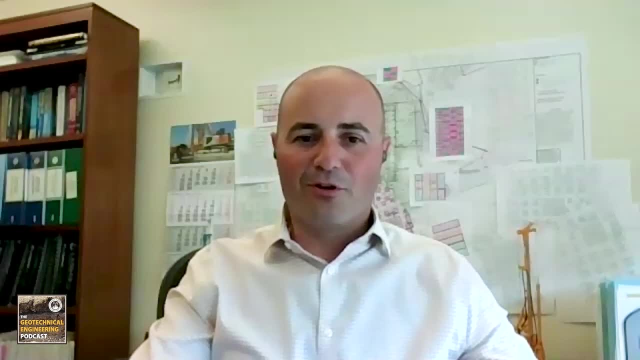 right, Yeah, Yeah, Some of our um internal programs were very helpful with you know why we do things a certain way, or how we do it, or just even standing next to the driller. Yeah, Um, it's a very different perspective. 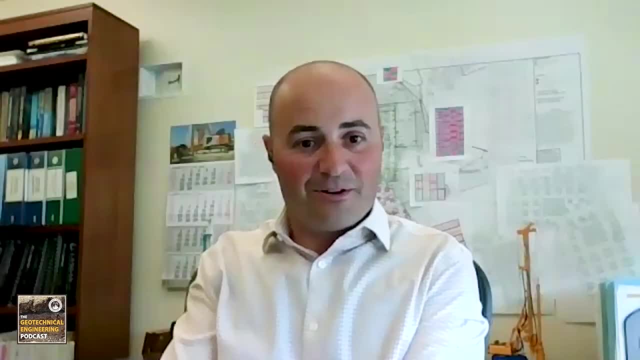 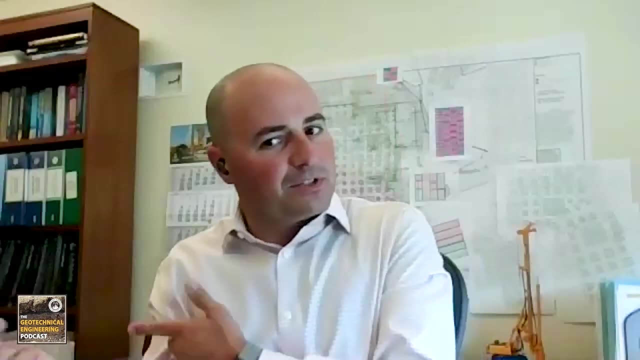 Like when I, when I came to work as a contractor and I went and stood next to the driller that was on the same payroll I was on: Yeah, Yeah, Right, Yeah. And I'm like, Hey, why do you do this? 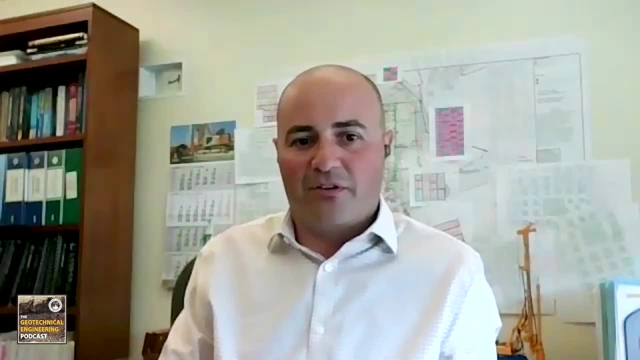 Why do you do, why don't you do that, Like you know things that, like you know, I I previously had a different opinion of before you know, and you know, there's, there's, there's. 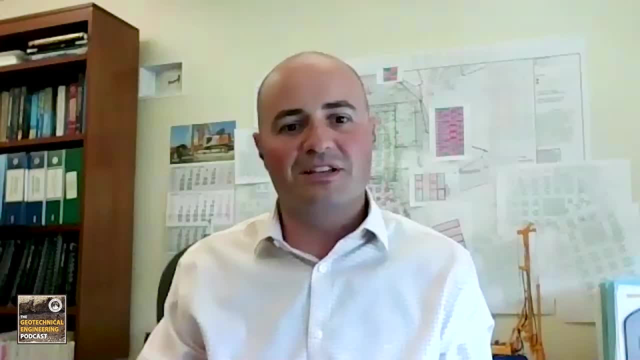 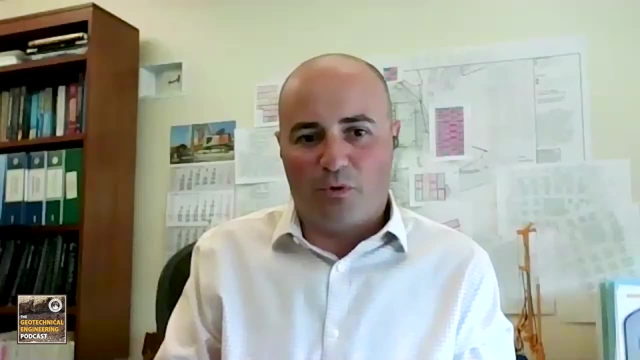 um, you know this is why we do this And and like it made a lot of sense, you know, to be able to get that firsthand perspective. Um, when you know the driller doesn't think you're someone who's trying to bug him. 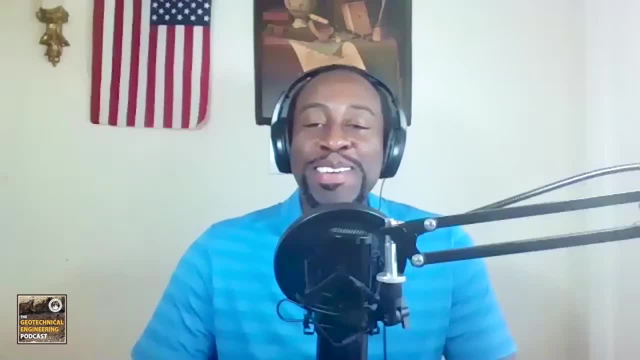 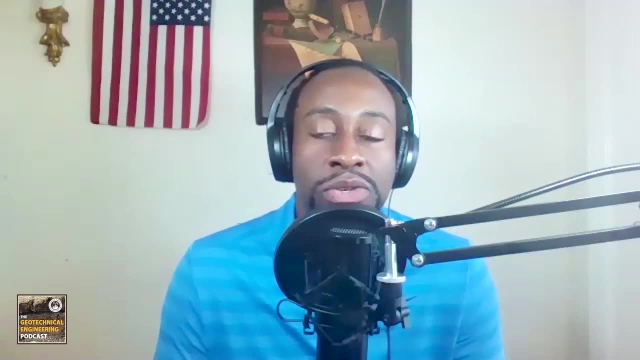 like your work together. Yeah, We're on the same team, same squad, right? Yeah, Oh, that's good And that reminds me, like soft skills, I mean a lot of what we learn in school, a lot of it's book smarts. 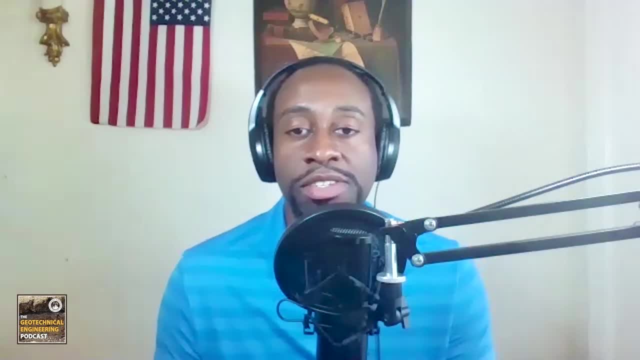 right. It's understanding the calculations, understanding the parameters, understanding the theory behind it. you may get an internship experience or a co-op and you get that practical experience, but soft skills are really important as you start to move up the ladder And 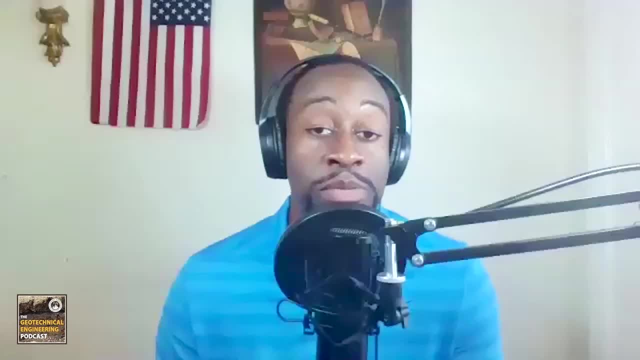 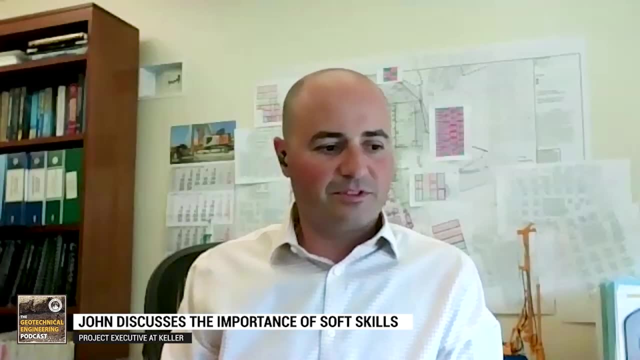 you know what would you say for how you learn those, and you know what it's meant for you professionally, Um, you know I've learned some hard lessons. you know I mean it's um you, you get to work on your approach and 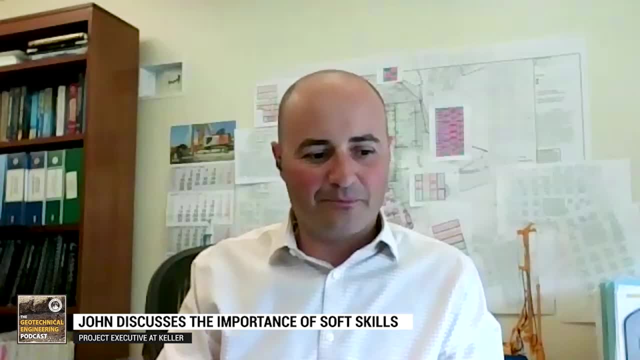 uh, learn how to lead a conversation and um, you know, and, and, and, to be empathetic. I mean empathy, I think is kind of. I have a word I use very often as a lead um, because 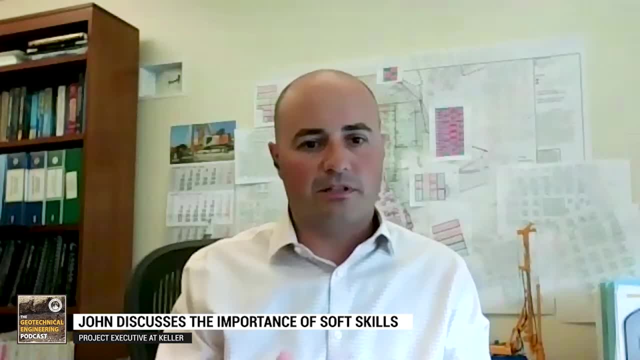 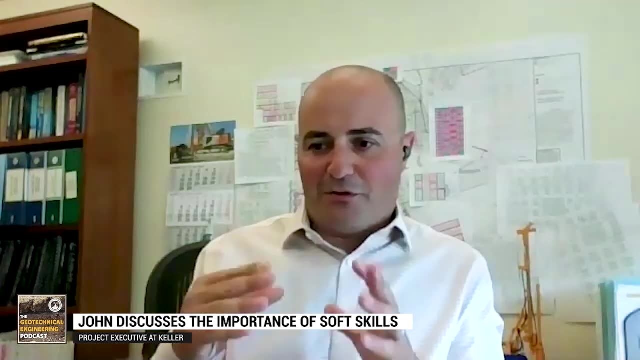 uh, you know it's, uh, you know, even say in a meeting with, like a developer or somebody this developer could be, if you don't and you have empathy for what they're going through, or like you know. 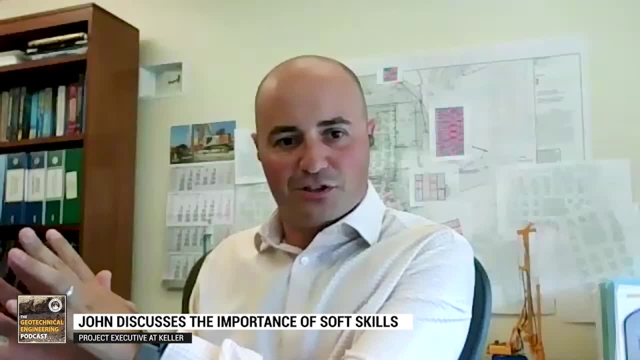 they know that if they have to go to a, a, a heavy duty foundation like the job's not happening Right. So it's like, okay, how can, how can I? I'm empathetic to what you got and 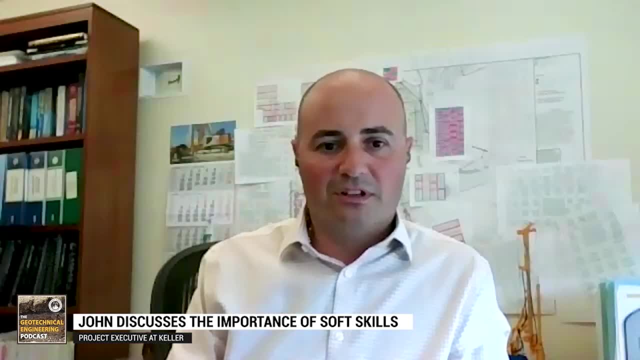 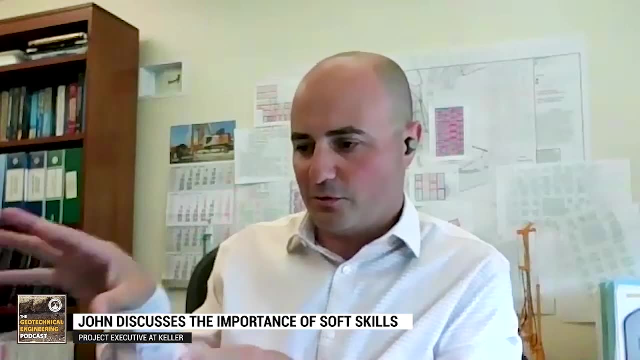 and you know I'm going to be here for you and and fulfill that role And um, and even even in general, like I I always kind of using that empathy is just just switching over to the um. 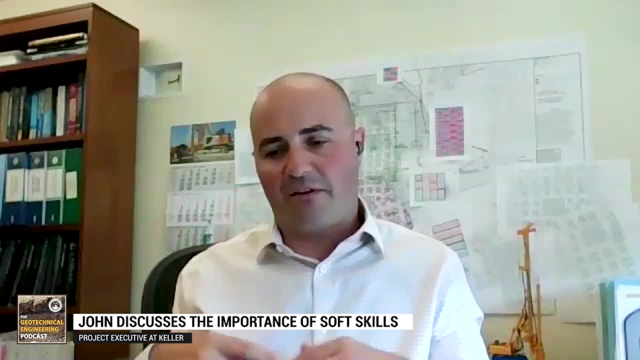 you know, just even in the office, and the different personalities, and you know, having empathy is good as well, but also understanding, uh, the other party's worldview, Like they have a view that they've built up with, you know. 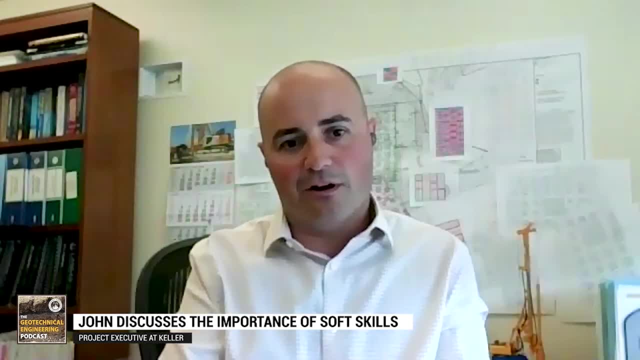 in their life, with you know the how they got to be where they are, And so there's a, there's a, there's a view and a perspective that that they come to the table with, And so being empathetic. 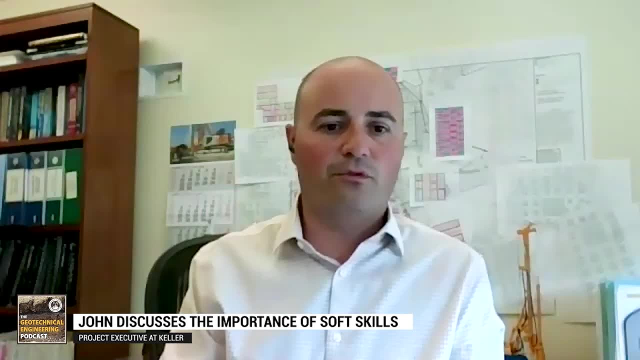 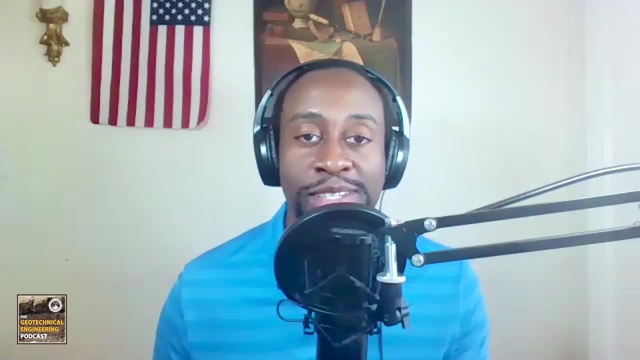 of where that may come from or why they may say a certain thing. it'd be very helpful in in leading or directing a conversation. It makes a lot of sense, I mean, if you don't take into consideration somebody's motivational values. 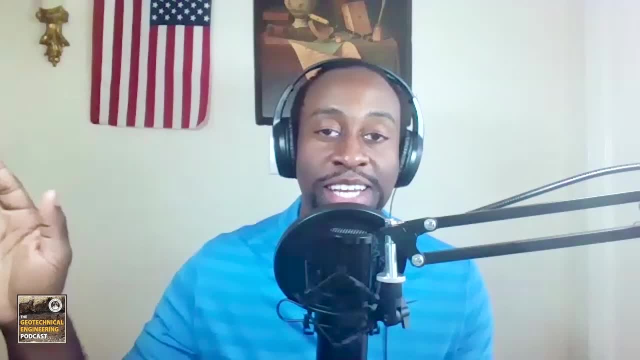 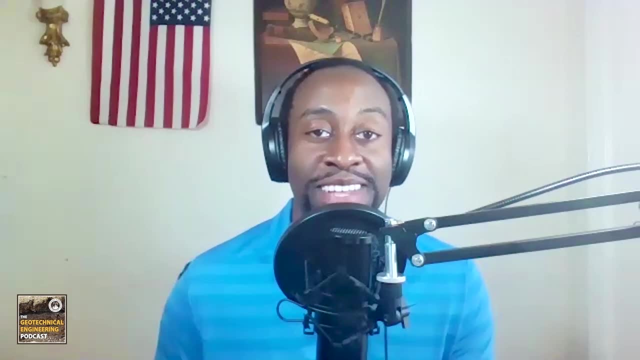 you could completely say something that kind of spends them in the wrong direction as opposed to encouraging them. So that's, that takes a lot of work And you know, I think that people think of engineers as not having that skillset right. 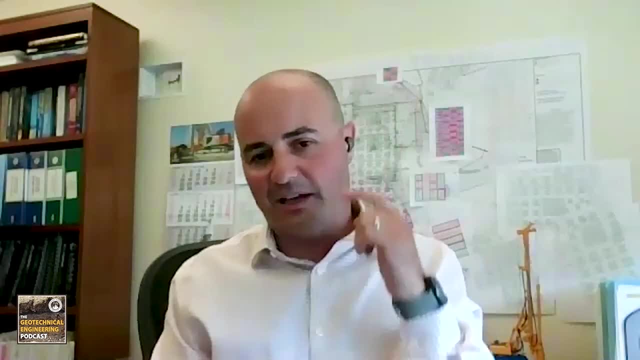 Yeah, I mean, you take that and you get some energy and enthusiasm and and, um, you know, and you you're going to have a couple of days stumbling, you know, and then all of a sudden it'll click a little bit and it'll get better, and 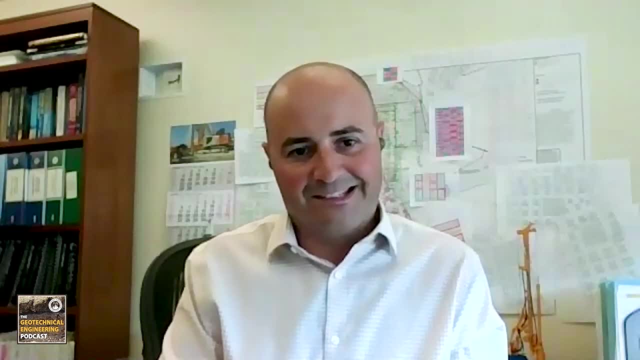 better. Um, just, you know, you gotta, you gotta, keep working at it. It doesn't, you know, you know it doesn't start on day one. No, not at all, Not even a week one or a month one. 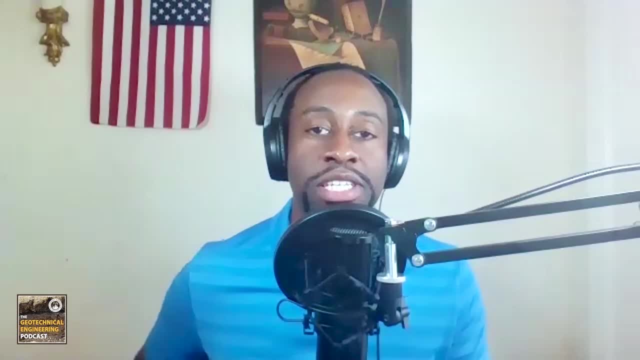 It takes. it takes some time. It takes some time. Now you think about your team and you know building your team. you know that relationship between the manager and the staff. I have to imagine that, um, there'll be some challenges. 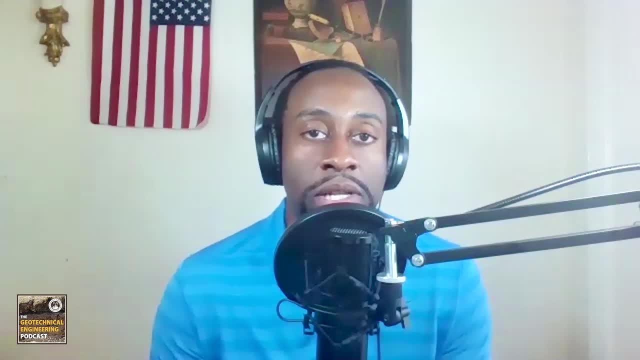 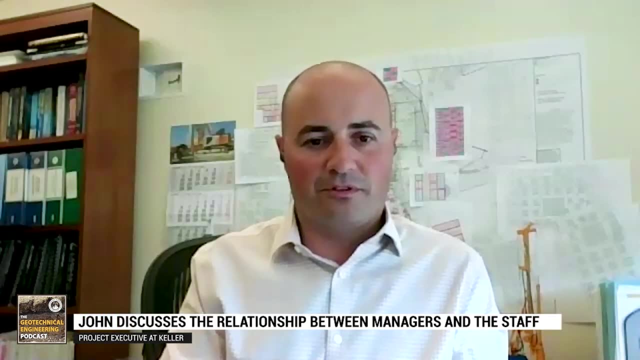 but I have to imagine there are some things that are really rewarding about. you know what that looked like. What can you share with the listeners? Yeah, So you know, the group of people I work with is great. I'm. 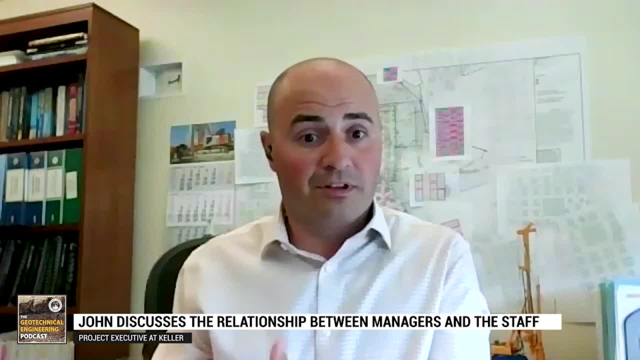 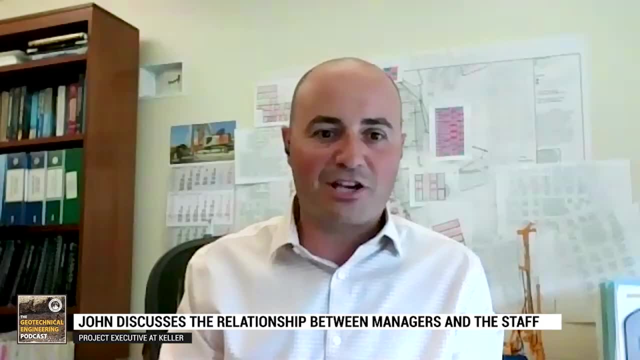 I'm fortunate in my position to have the people that I work with. You guys are a lot of fun. Yeah, You know what The, the, the group that I'm working with right now. they're, they're, they're into it and they have passion and drive and emotion. 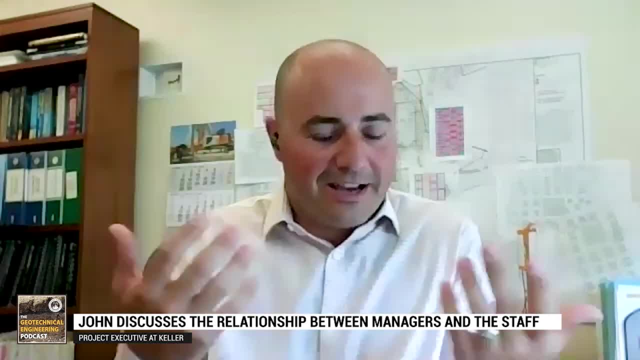 which, which, which works good, because I have that stuff too, Right, Yeah, You know, it's like a: we build each other up and it's nice And, like you know, I feel like my job is to kind of raise them up and like give them the 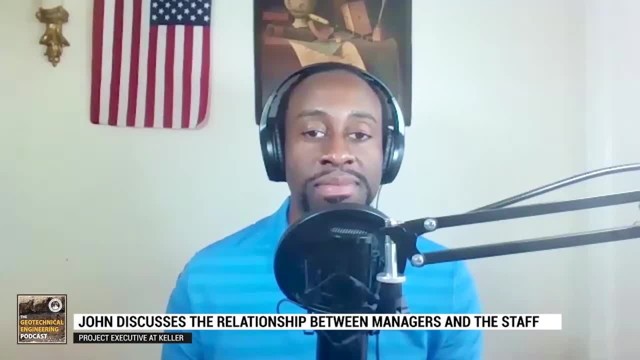 confidence, the confidence to make the decisions they know how to make. and you know and like, grow as a team, Cause you know, every time there's a new job, we're all learning something new. Yeah, That's true, You know. 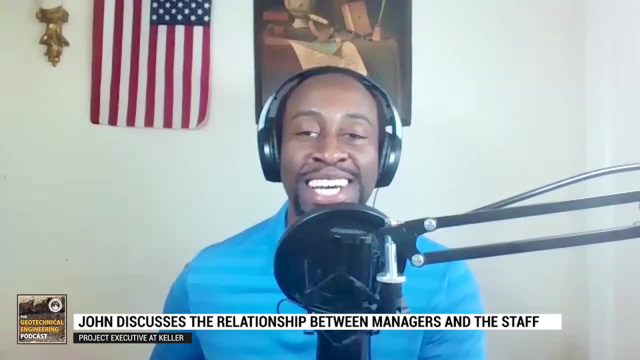 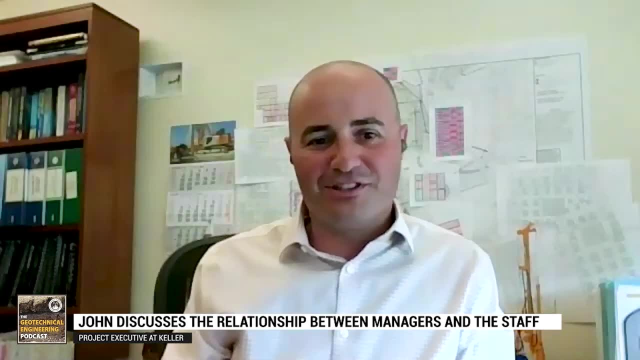 I've never done the same job twice, Me neither. It's the benefit of geotech, right It's, you know it's. it's every. every job's a new opportunity to do better than the last one and learn something new. 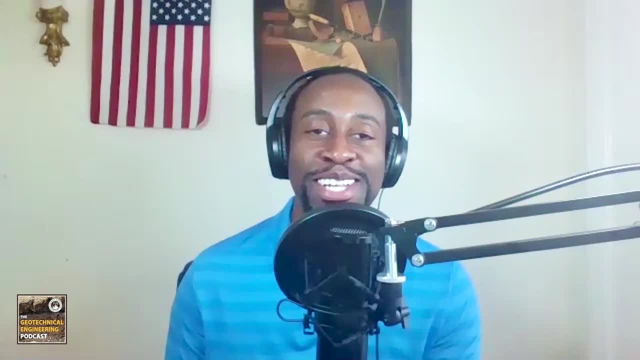 Right, There you go, You can be across the street and it's like, Oh, it's totally different here than it was over there, Not what I expected. Yeah, Exactly, That's why they call it practicing geotechnical engineering. 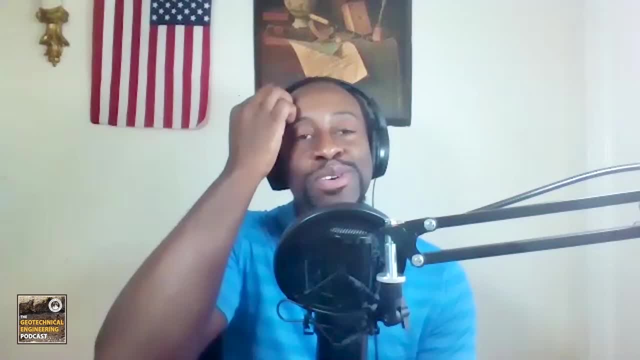 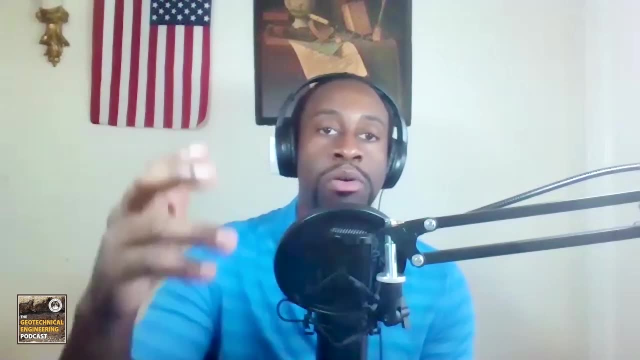 right, Yeah, Yeah. What advice do you think you could give for a geotech that may be considering a move from, say, like, a staff or senior staff level, moving into management or more leadership roles? What advice would you share? You know, don't. 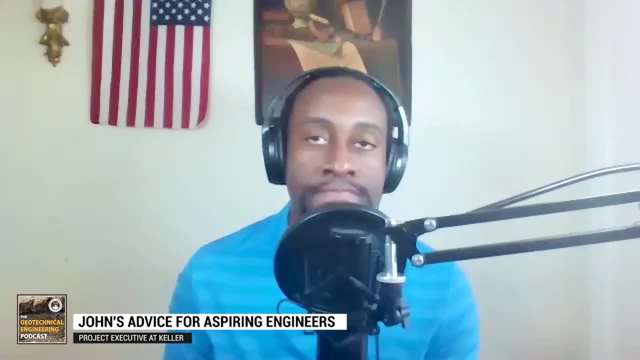 don't be afraid to take a chance, Like a little risk is okay. You know calculate your risk, understand. you know what your benefit, what your benefits could be. You know one thing I learned once was not call it a negative. 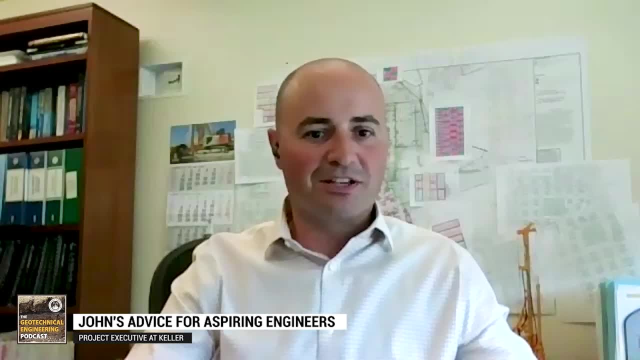 call it a Delta: get your pluses and your deltas. So understand your pluses and Delta. do your own analysis and understand which way it can go. I mean work hard, keep your nose down, learn everything you can, Because I think part of being 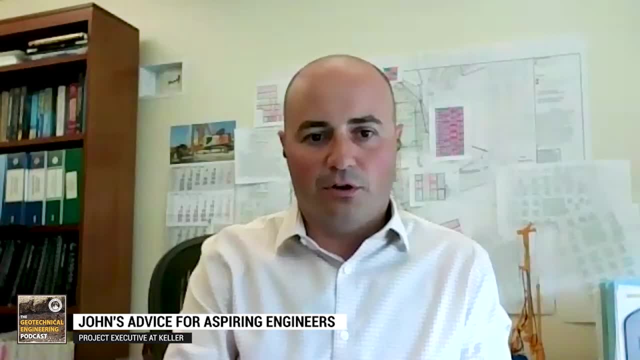 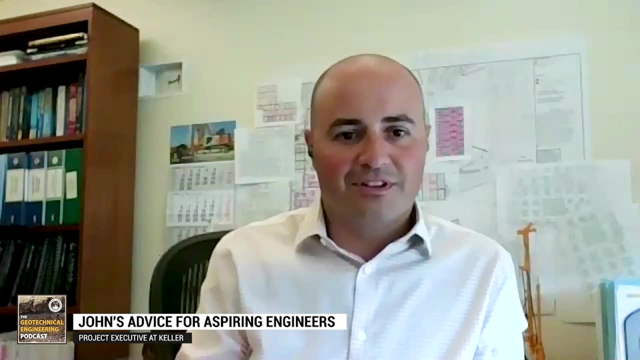 you know, getting to that managed managerial role is, you know, having the. besides the technique, you have to, you have emotional intelligence, technical intelligence and you need to use those both. Um to uh to uh. 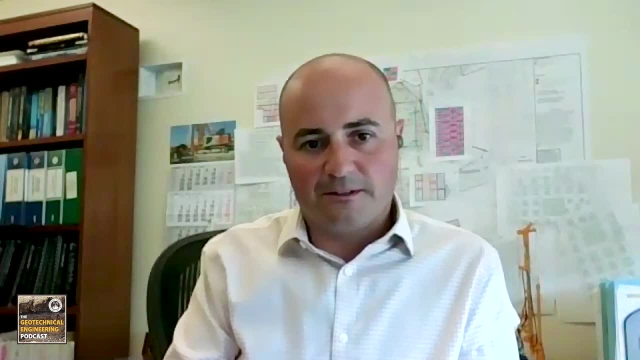 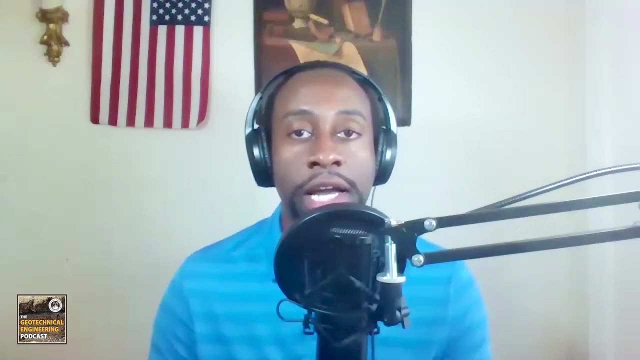 to put that team together and put the right people in the right spots. Excellent, Excellent. I know that throughout your career you've been pretty active in, uh, the professional societies. Anything you could share there as far as how to get more involved or why one? 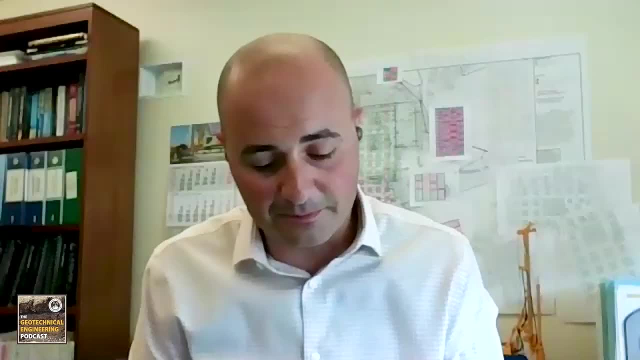 would want to be more involved. Yeah, So I mean, that's um, that was uh. it's always like a near and dear place to me. the professional size I mean. you and I were on a committee together once upon a time. 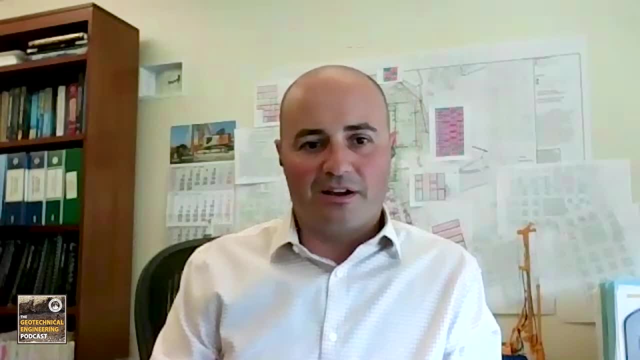 And, um, really, you know the societies that you know, uh, you know that that meant a lot to me. I, you know, I, I went to their events. Um, you know, I, I know that they look for different people to be on their board directors or 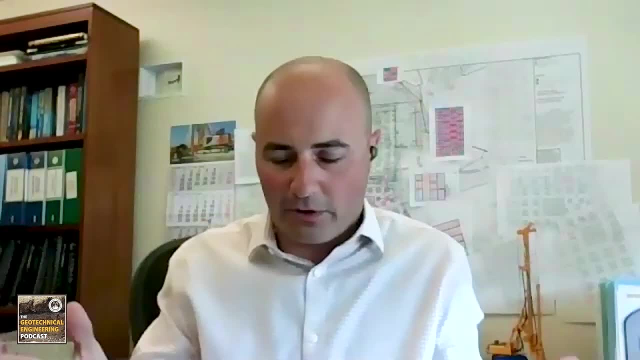 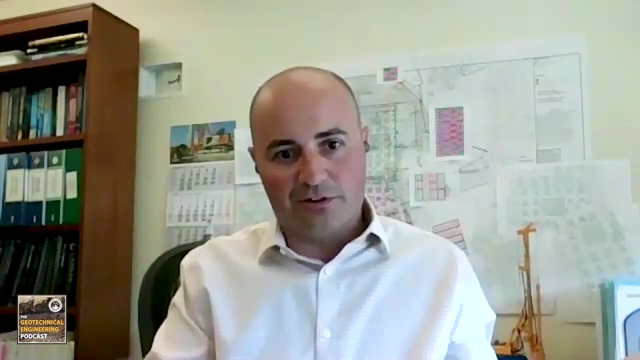 their or their officers of the or the committee, whatever they call it. And, um, you know, when I heard there's an opening coming up, you know I started talking to the current leadership and saying, Hey, I'm interested. 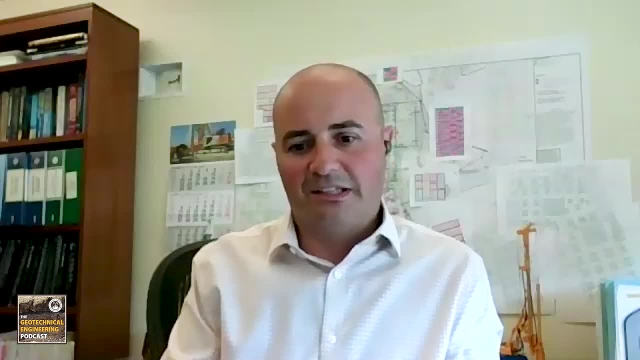 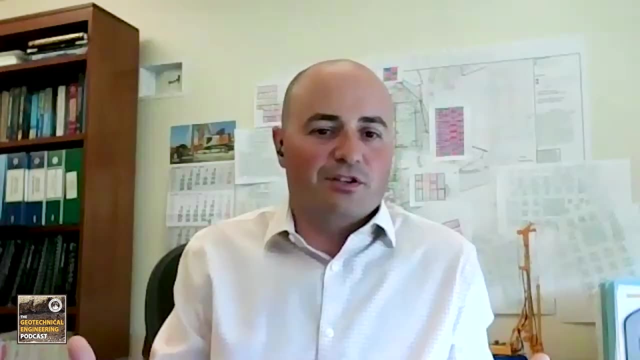 And you know, when you kind of work your way in because you know I, you know, forget that I work for for Keller I. I love working for Keller. It's a great company, but I love this industry. 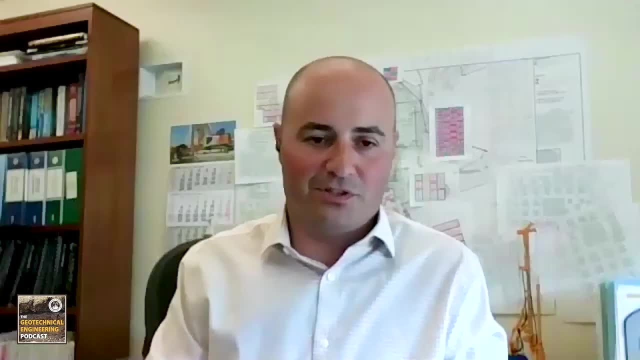 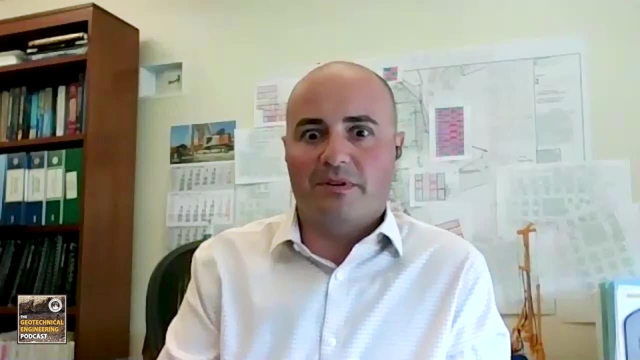 you know and like, and I want to see the industry be better also. Yeah, You know, And so it's, it's, it's. I think it's a great thing to uh be part of something besides um. 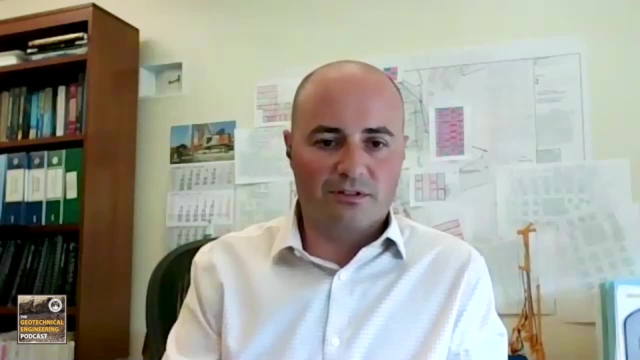 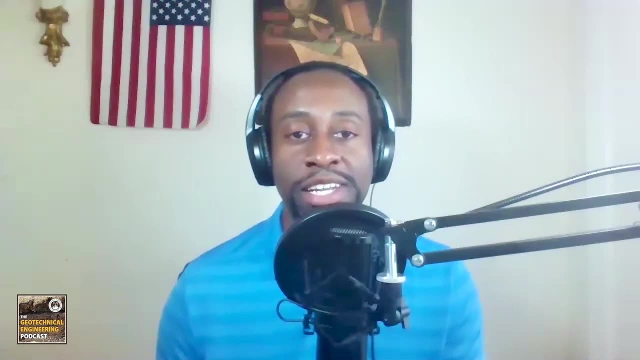 you know just your company, you're part of the industry, you know. Yeah, I think that's really powerful when you think about it, Cause you know we were in class and we're learning about what it means to be a geotechnical engineer. 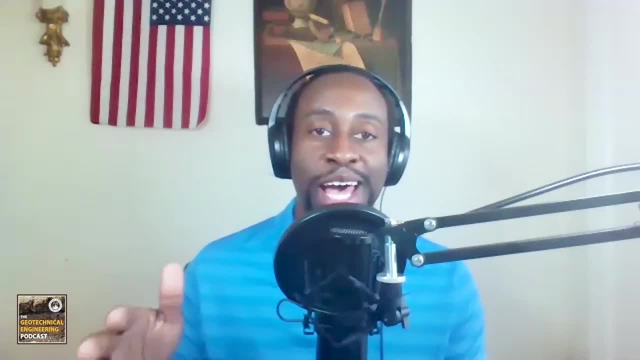 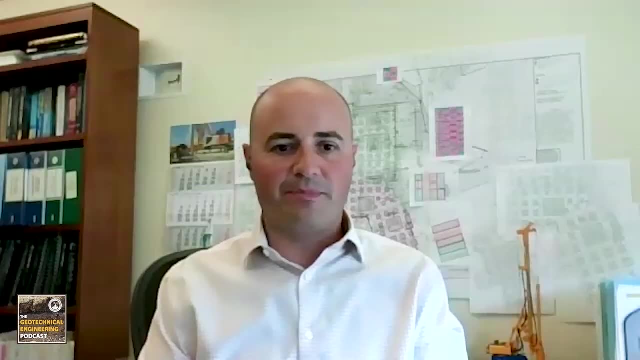 And then, after you do it for some years and when you're a part of of actually making the industry better, there's something really powerful about having that opportunity. you know- Yeah, I mean listen- you meet a lot of great people on the road too. 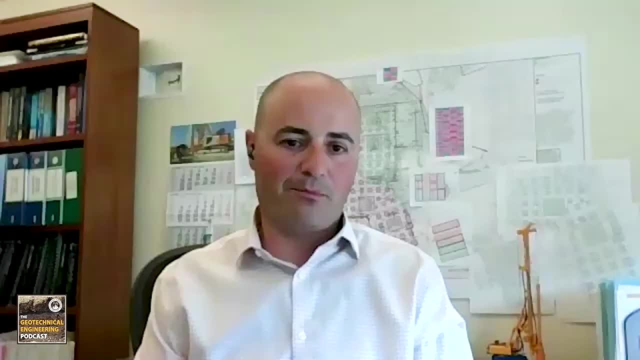 I mean, I mean, you work with a lot of great people, I'll work with a lot of great people, but uh, there's a lot more of them out there. There's a lot more, That's true, Yeah. 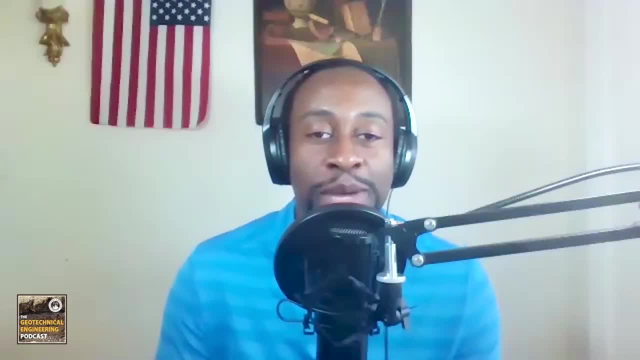 Oh, that's great. That's great, All right. Well, we're going to take a quick moment to take a break, and we're going to come back just after a moment and we're going to finish this up with John, as we have our career. factor of safety in segment. 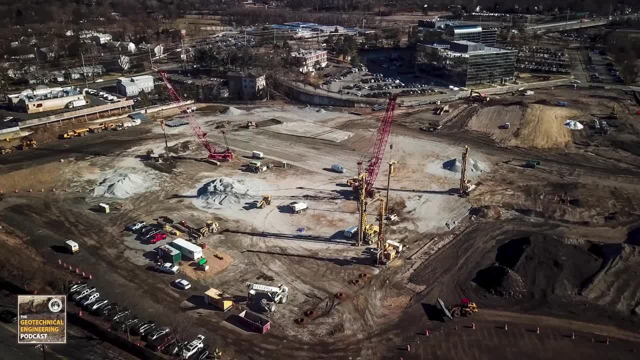 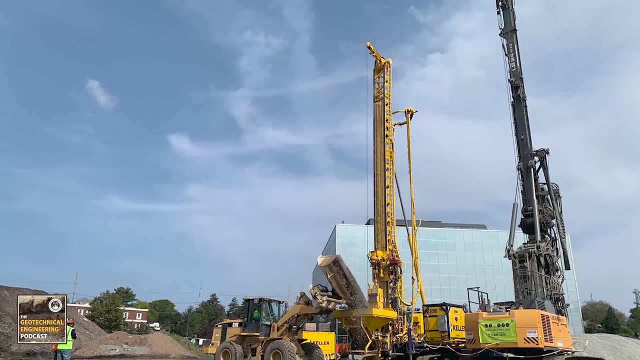 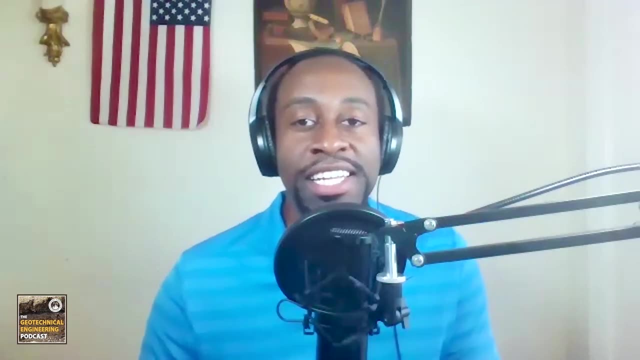 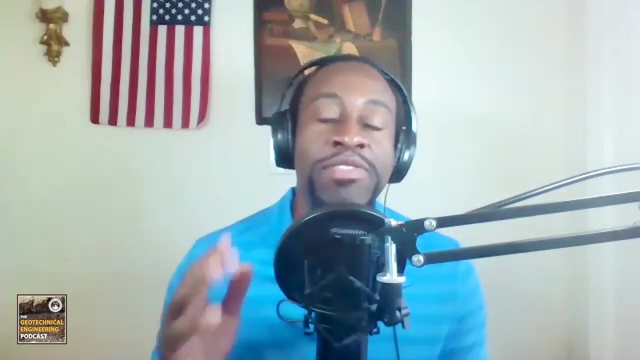 stick around. Welcome back. It's time for our career. factor of safety in segment and geotechnical engineering. just like many disciplines of engineering, it's important to incorporate a factor of safety into your design, And we talked about that a little bit today with our guests. 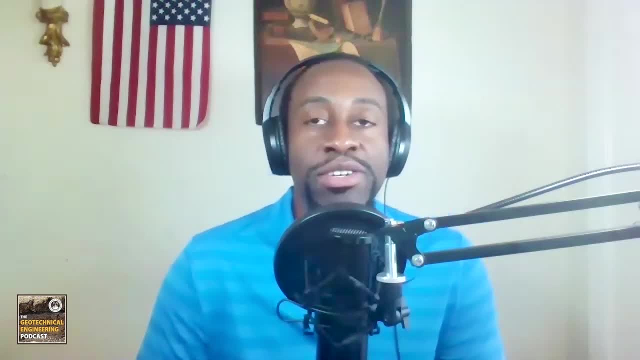 but what about incorporating a factor of safety into your design? And what about incorporating a factor of safety into your career? today, Of course, we're speaking with none other than John Grillo P E. John, the work that you do involves a lot of risks, to both you and your staff. 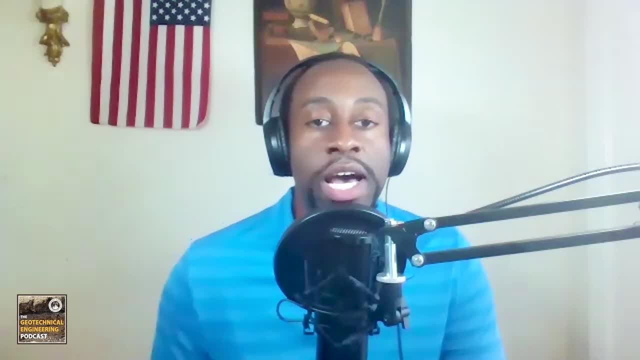 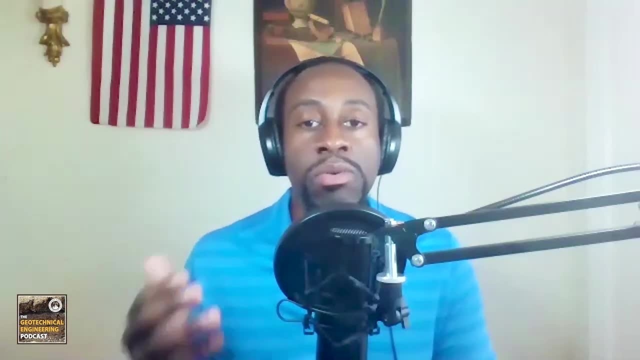 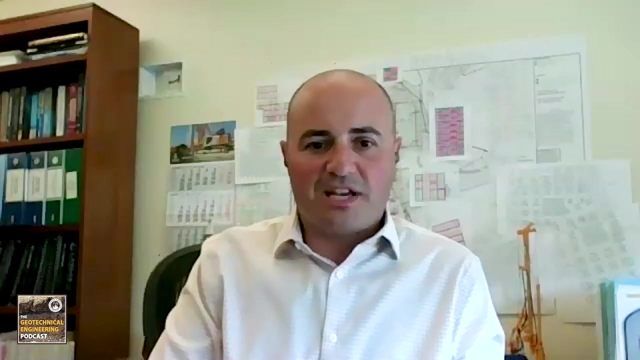 as well as to the community In some sense? how have you built a factor of safety in your career, as well as those that you manage to give yourselves a factor of safety and working on construction sites as it relates to safety? Um, so the factor of safety for safety. 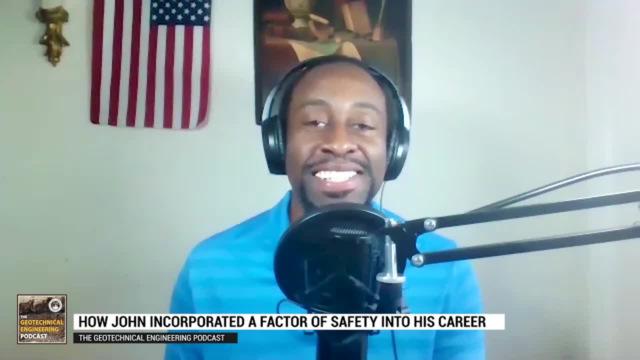 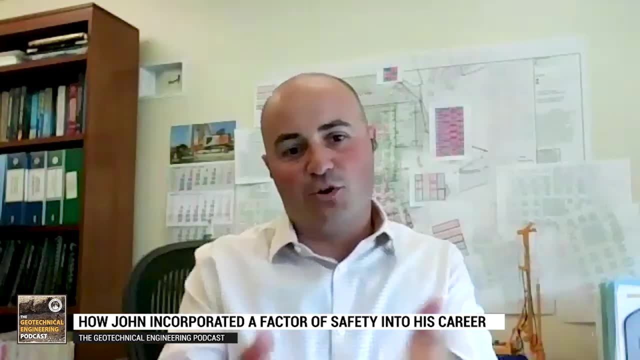 uh, should be pretty high. Uh, one thing that, um, our safety team says pretty often is: let's go from I think it's safe to I know it's safe, you know. and that really sticks stuck with me because 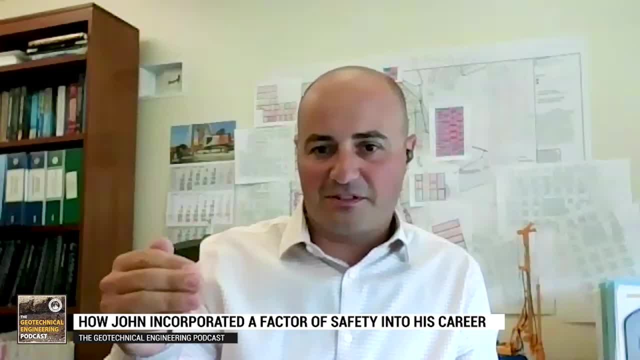 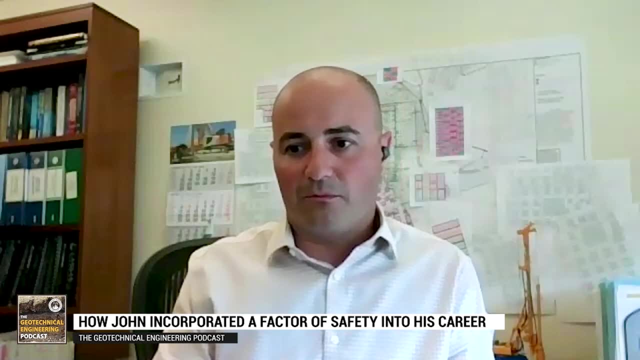 you know this, this, this industry is awesome. It's also dangerous, Okay. So, um, I think it makes sense to know what you're doing is safe. Yeah, You know on the job site, do do. 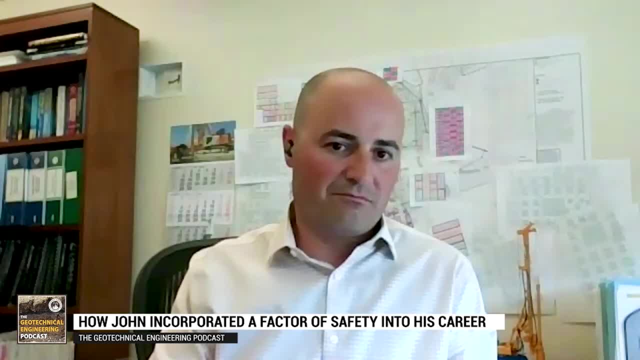 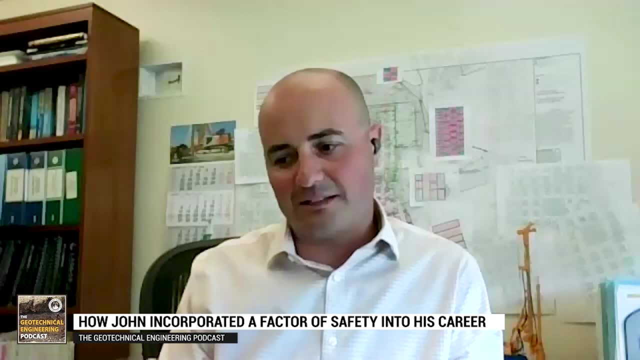 did we, did we? uh, it was secure, the load. Um, how are we picking this tool off the truck? Like, is that, is that safe, You know? like that's you know I? I think that's totally worth even the extra minute you need just to check. 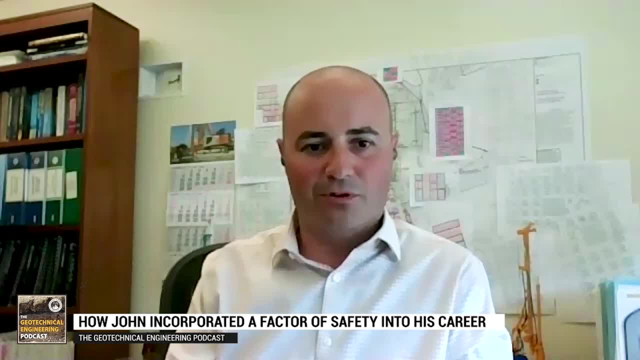 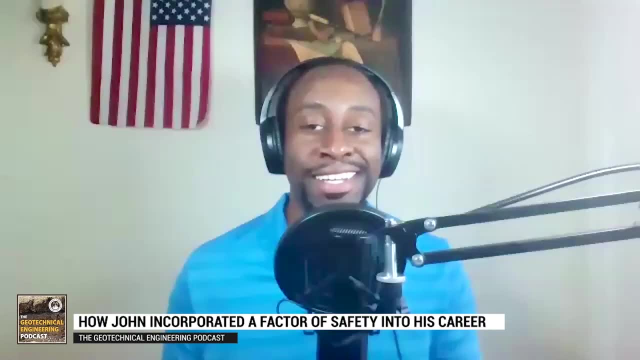 check the rigging And that's, and that's. that's to me a very, a very simple thing. that is always like: Hey guys, take your time. It's really hot today. Guys, drink some water. It's important to do those things. 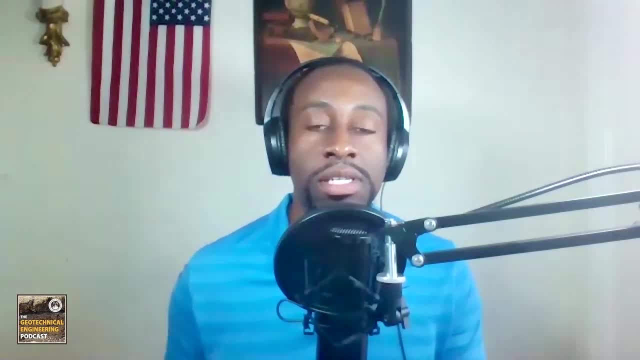 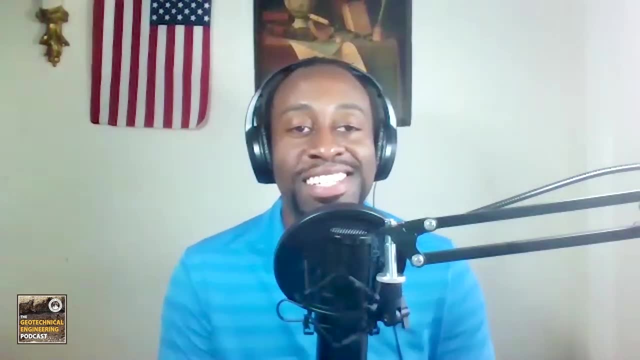 Makes a lot of sense. It's usually when uh folks are cutting corners that that uh something silly happens And, like you say, it really only takes a moment to just think about it. Right, That's great Well. 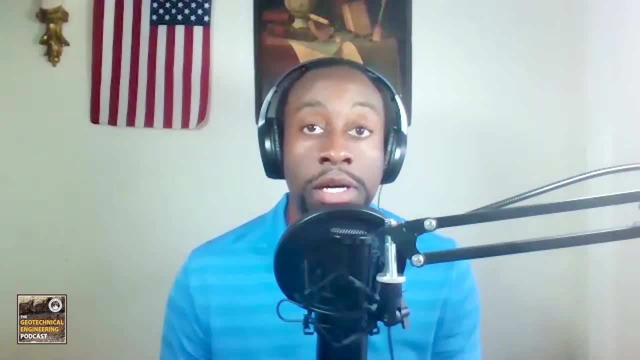 John, thank you so much for coming on, Thank you for sharing all the great insights that you did with um uh with this talk, And thank you for your service to the industry. We really appreciate what you're doing for the engineering community. 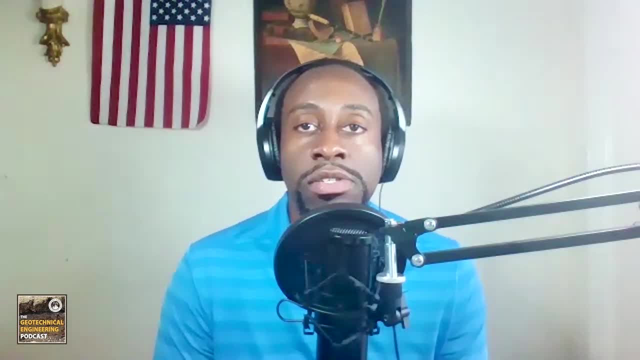 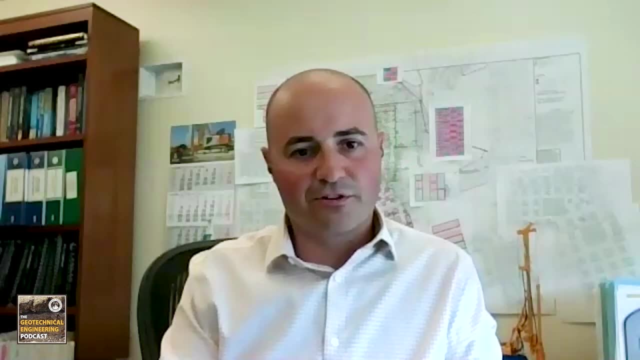 Now, if somebody wanted to reach out to you, what's the best way for listeners to reach you? uh, social media or email address? Yeah, Email is great, Uh also. uh, LinkedIn is great as well. Those are. 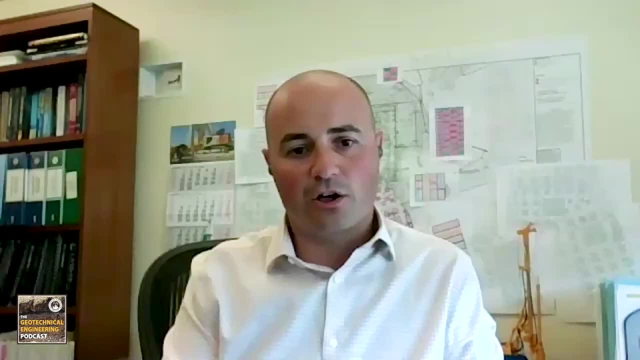 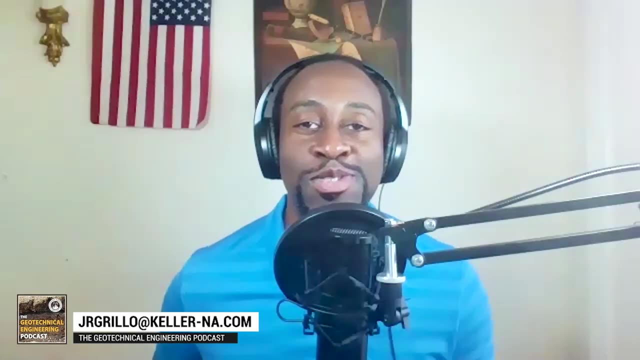 those are probably the two best ways to contact me. Okay, Excellent. What is your email address? So my email address is jrgrillo G R I L L O at keller-nacom. Excellent, Excellent. Thank you so much for being here.